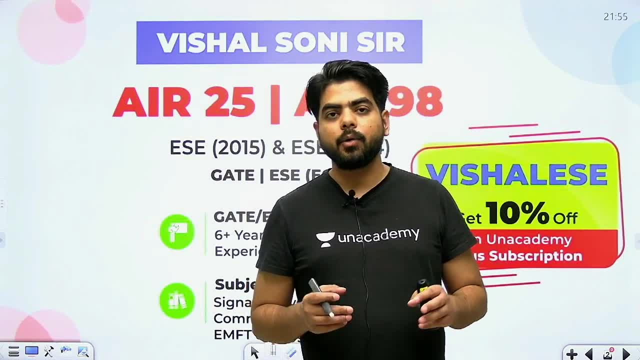 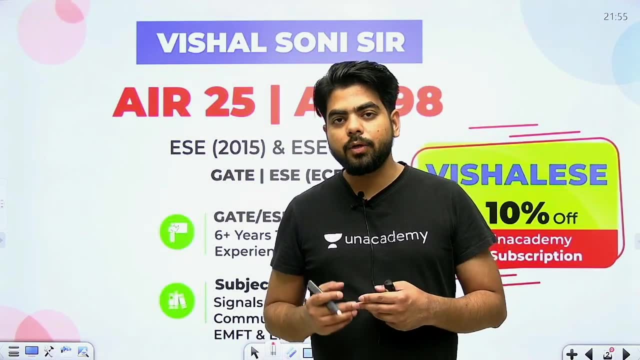 teaching on Unacademy and I really feel proud to be the part of the Unacademy team, because Unacademy is the revolution in the field of free education and in the field of affordable education, And we as a team are really looking forward for every student to just come on. 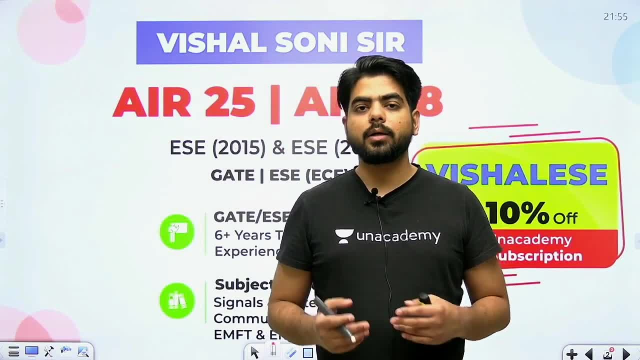 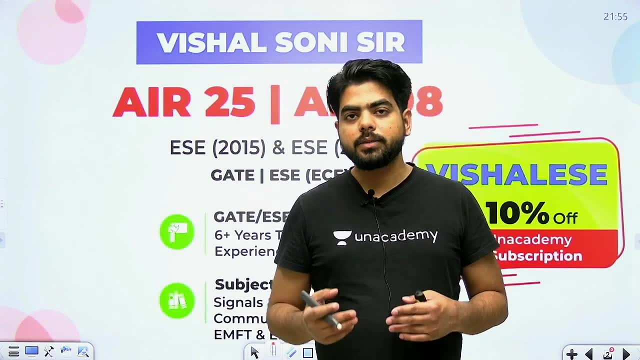 to the Unacademy platform, You can attend the special classes, you can come on to this YouTube channel and you can stay connected with us so that you can understand the quality education and you can understand the efforts that we are putting in so that every student 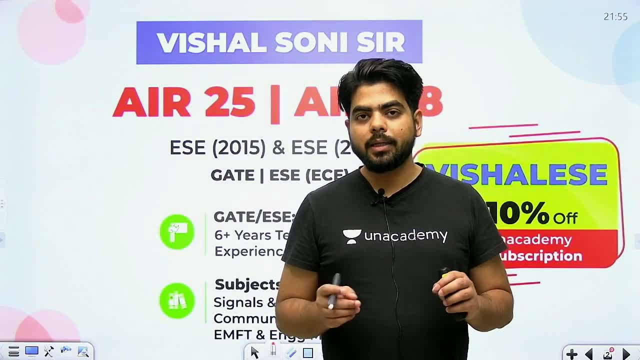 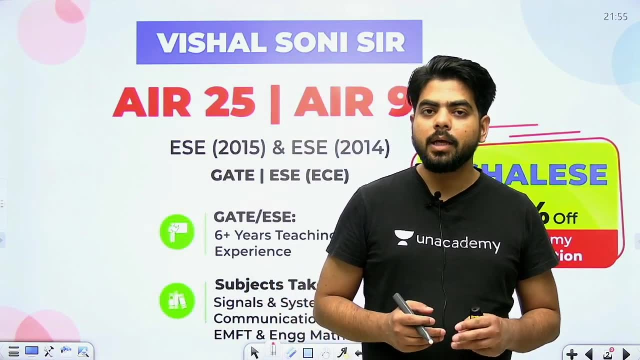 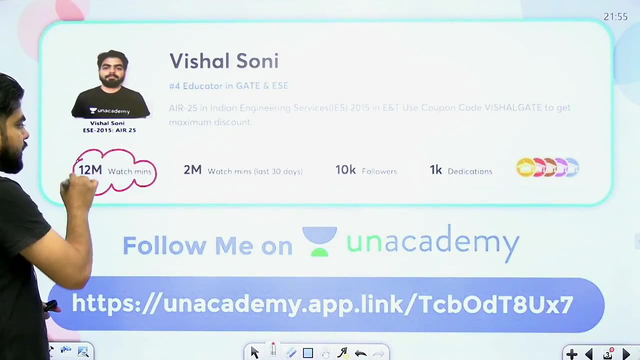 of this country, whether he stays in a village or he stays in a town, should get the access of the content- that too, in a very affordable prices, And he can also- or she can also- clear the examination with the best possible ranks. So right now I'm teaching on Unacademy with more than 15 million watch minutes in the 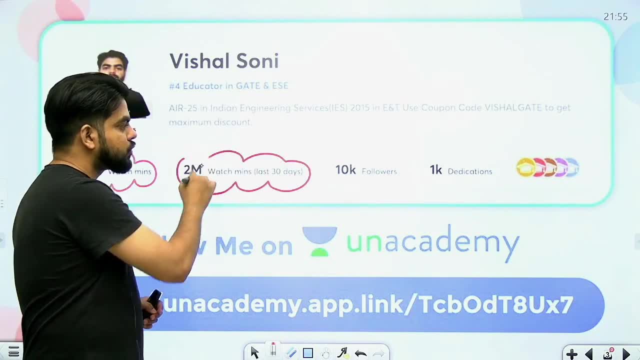 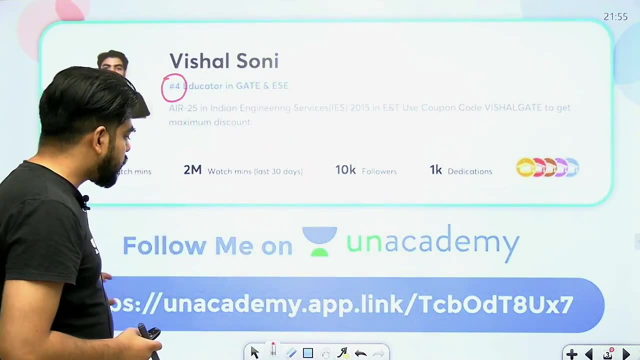 overall duration and 2 million watch minutes in the last 30 days. So I am right now the top educator in Unacademy across all the branches, having ranked 4 right now, And you can also follow me on Unacademy on this particular link, So you can go and follow me on Unacademy. 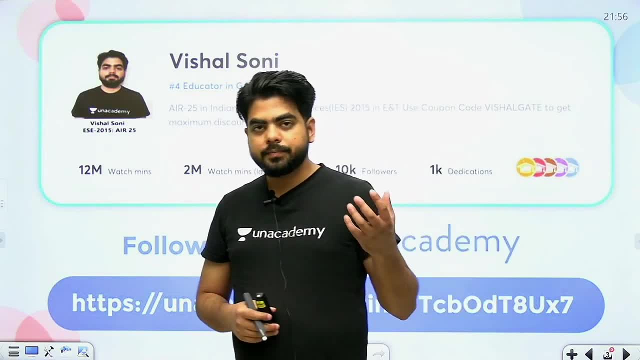 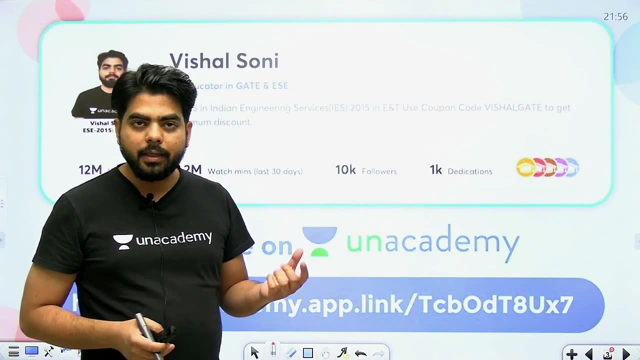 Apart from that, my advice to every student is that you should not be a student of the pageati channel. How should you crack the examination and what are the components to cracking the examination? So the first question that comes to the mind that: can anyone prepare? 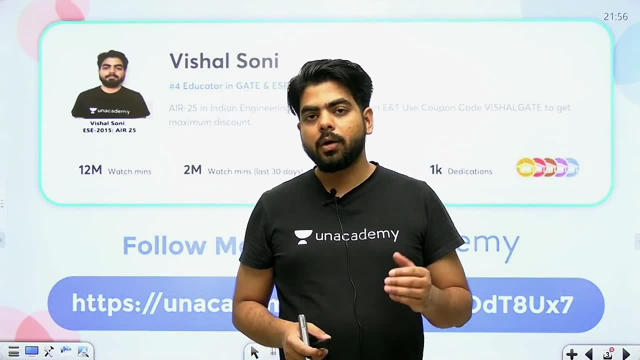 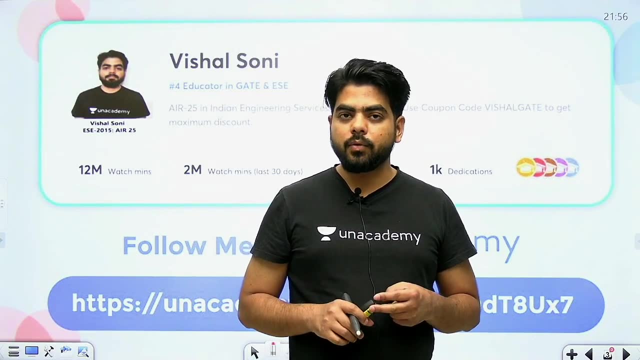 from the YouTube. Yes, you can prepare from the youtube, but you should develop or cultivate some habits in yourself. For example, you should be very much disciplined. You should arrange the extra resources, For example the PDFs. you have to arrange the test series. 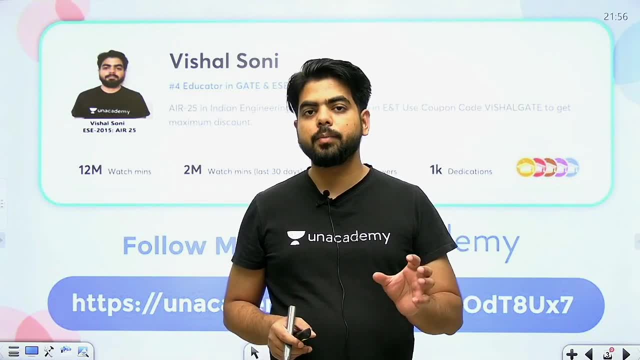 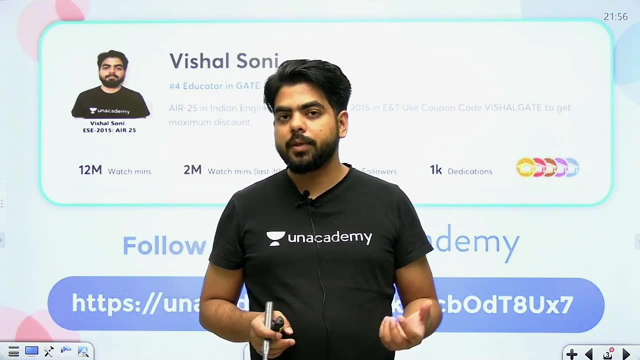 you have to arrange by yourself And, most importantly, that self-discipline you should be containing in yourself so that you can be in a very corrective manner And you can approach the examination in the best possible manner. so all these things you have to arrange. 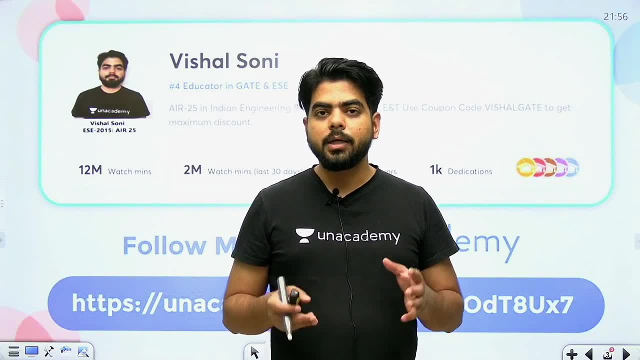 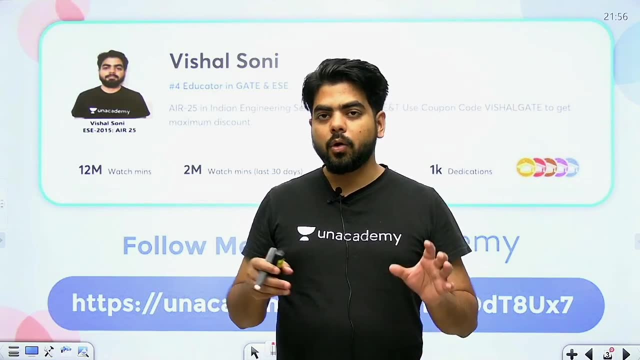 yourself the sense of competitiveness you have to cultivate in yourself, because the audience on the youtube are not that much of competitive in nature, or maybe you cannot feel the competition which is present right now. so all these things are the part of the journey if you want to prepare through the 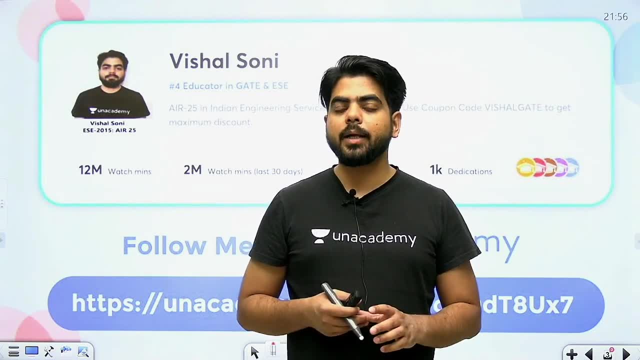 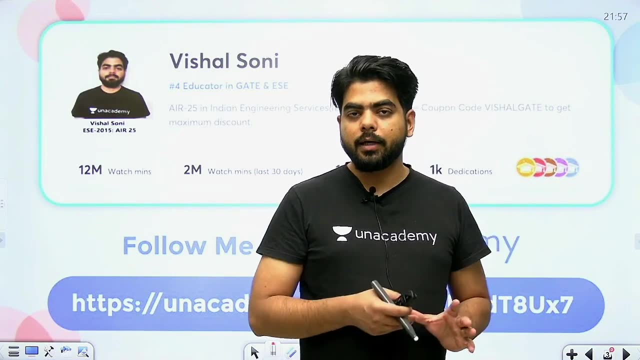 youtube or maybe, if you want to prepare, through the free resources. apart from that, if you want that you should get complete content, then this is the youtube channel. on this youtube channel itself, all the free content are available. you just have to go to the playlist. all the subjects are. 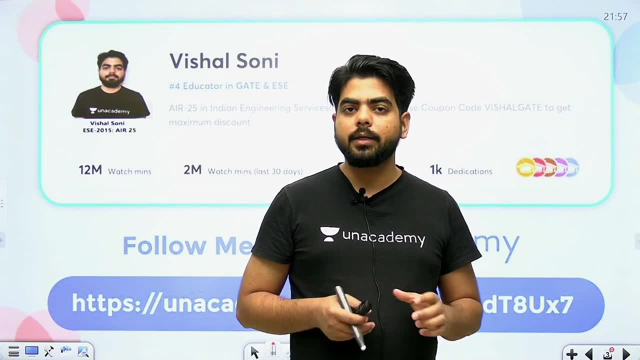 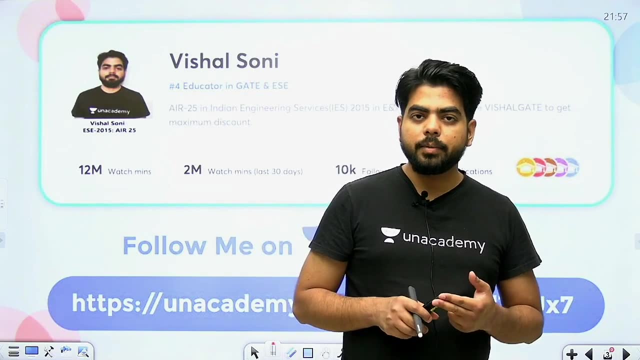 completed there. you just have to go and watch all the lectures one by one- definitely will be getting benefited, but the extra things that i have told you, that the self-discipline and the sense of competitiveness and a lot of things you have to arrange by yourself if you are comfortable in that. 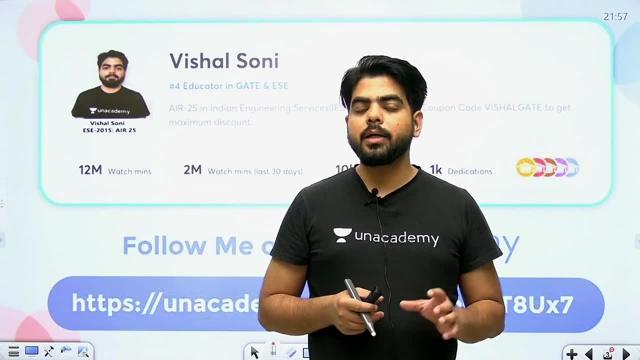 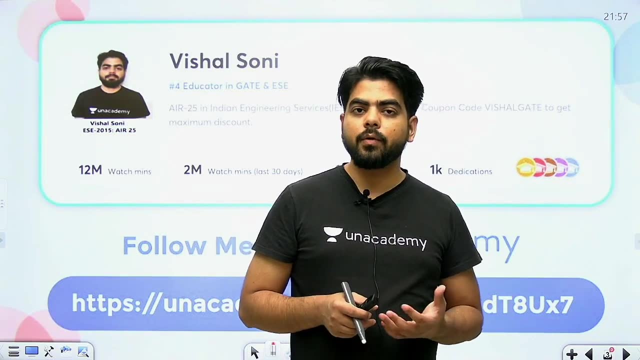 then you can do that. apart from that, you should also have an academy learning app so that the special classes you can attend. a lot of educators in this country are actually providing the special classes- that, too, absolutely free of cost, so that you can get the quality content in the best possible manner. apart from that, there is also another. 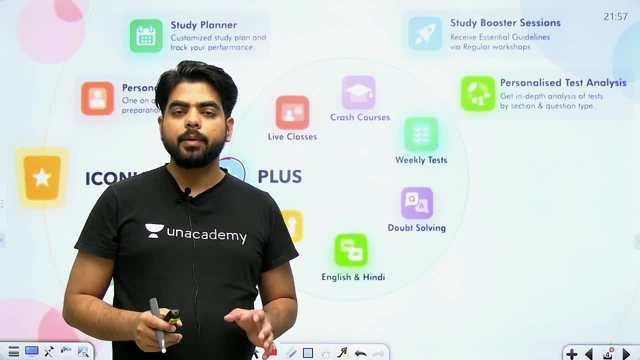 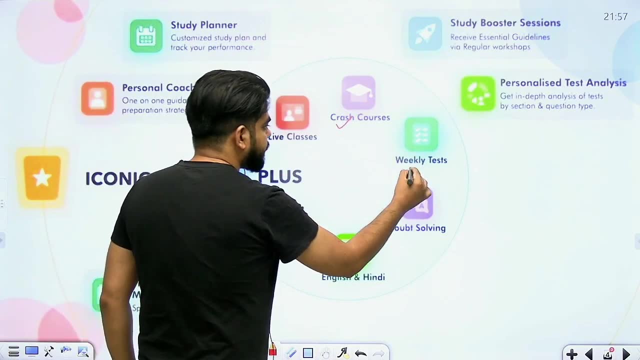 component for you which is an academy plus. so, on, an academy plus, what is your job? you just have to study. if you join this, an academy plus, you do not have to worry about the crash courses, weekly test, doubt solving sessions, the language barrier, rank improvement, batches, live classes, so all these. 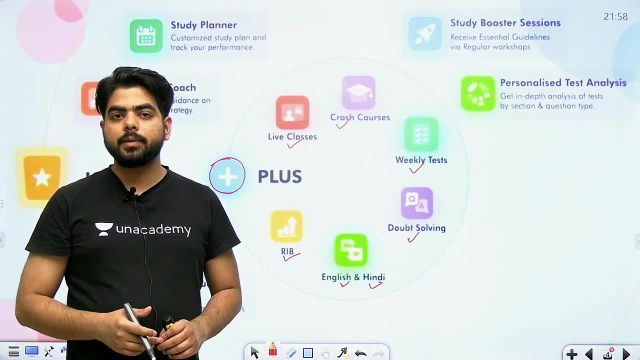 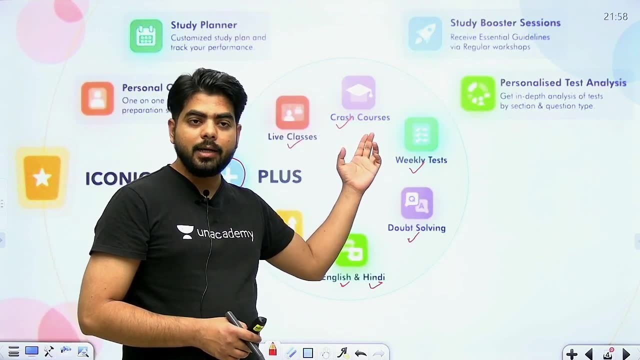 things will be taken care by an academy. you just have to take the academy plus subscription and you have to come on to that academy. You will be daily getting the live classes. you will be getting the crash courses when. you will be getting the crash courses when the syllabus are completed. 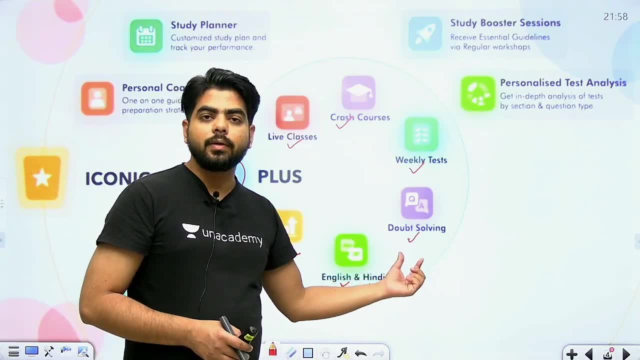 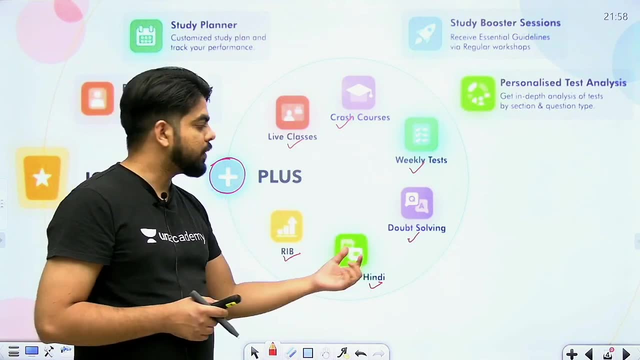 You will be getting the weekly test in the form of quizzes. Every fourth class is the doubt solving session, which is the major major, you can say the component or the major major impact will be creating on your studies will be this doubt solving group, Because until and unless your doubts are not being cleared, until and unless you are not. 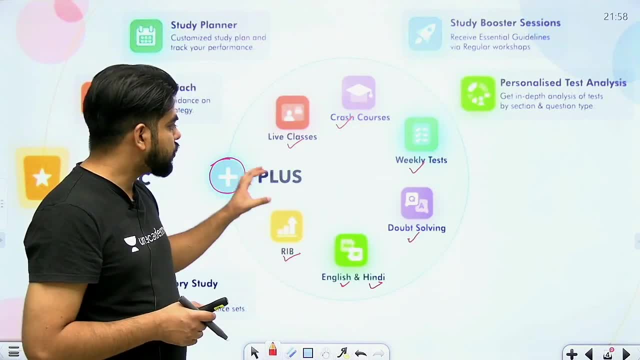 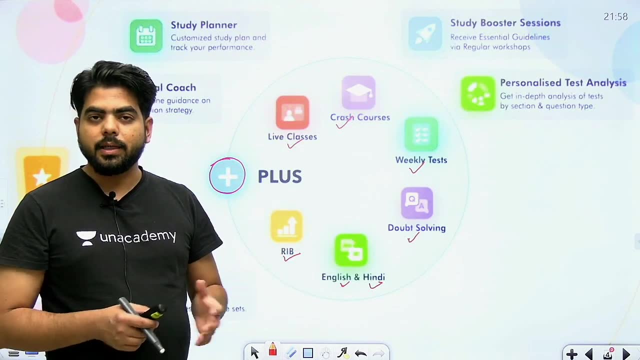 able to clear your doubts, you will never get the confidence in the subject. So once you come on to this, an academy plus every fourth class is doubt solving session. Apart from that, various other doubt solving sessions are going on. So ultimately, you will be getting your doubts cleared and you will gain confidence in the 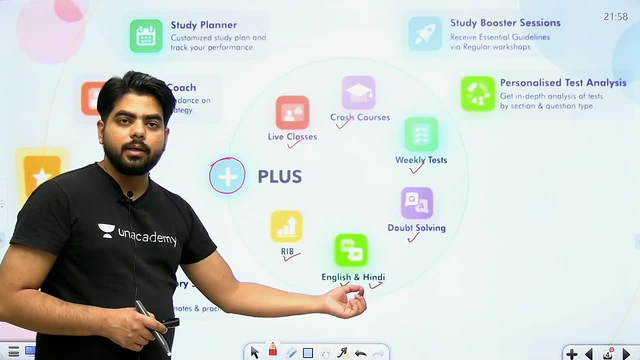 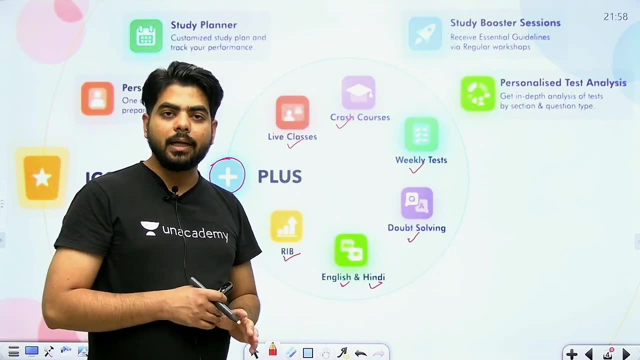 subject. The language barrier will not be an issue because the batches will be running both Hindi and in English, and rank improvement batches will also be there. So all these things are the component of this plus subscription. Once you come on to this, an academy plus, you do not have to be worried about your self. 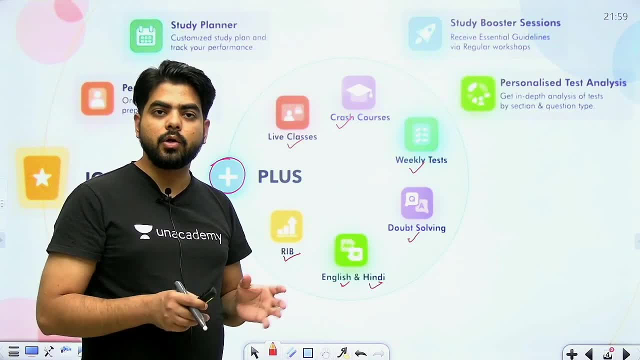 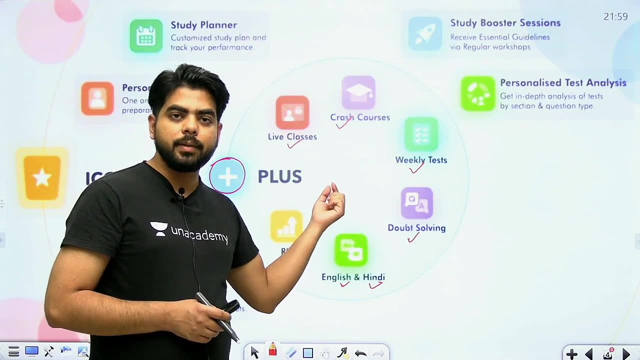 discipline, your competitiveness, nature- everything will be present on an academy because a lot of other students will be there. Since the classes will be live, you can also watch it recorded later on. So the discipline automatically comes, because you get the idea that you will be having the 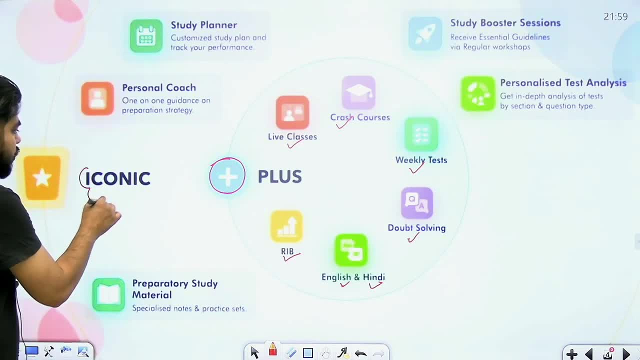 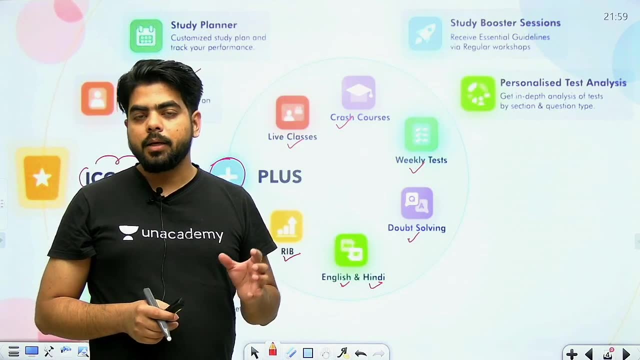 daily live classes. Apart from that, there is also one iconic subscription. in this iconic subscription, the game changer is this personal coach. So this subscription is for them. who thinks that their basics are weak, or those who are talented, but they need a continuous push. 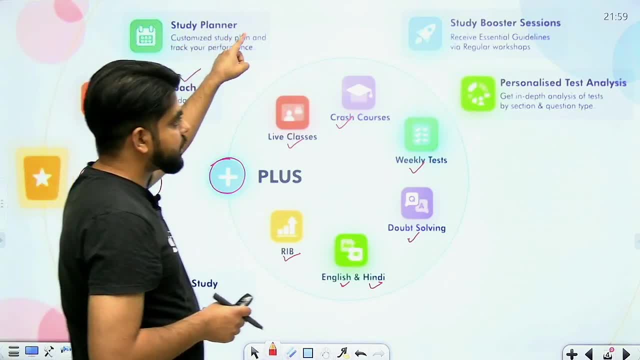 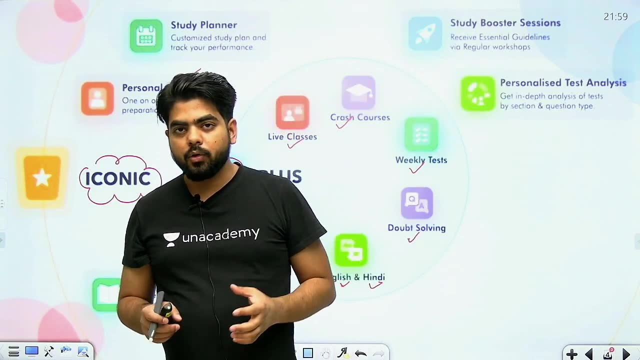 So this personal coach will be guiding you throughout your study. he will be giving the study planners. you will be getting the study booster sessions. Once you will get the test, you will be getting the analytics. analytics plays a major role in improving yourself. 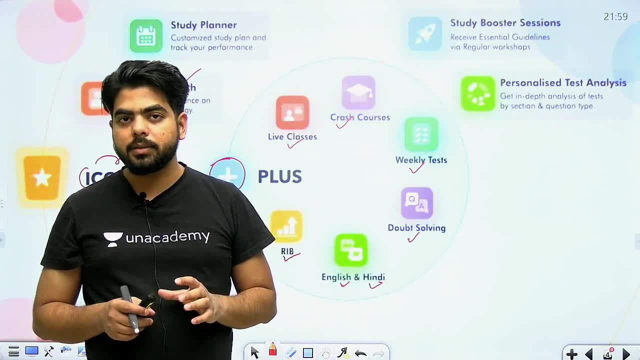 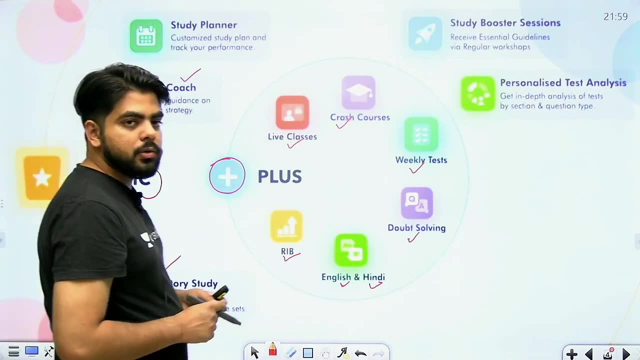 We, as a teacher, also get our analytics so that we can improve on the daily basis. So once you start getting the analytics, you will be also improving massively on a daily basis. Apart from that, there will also be the guidance for the mains once you clear the claims and 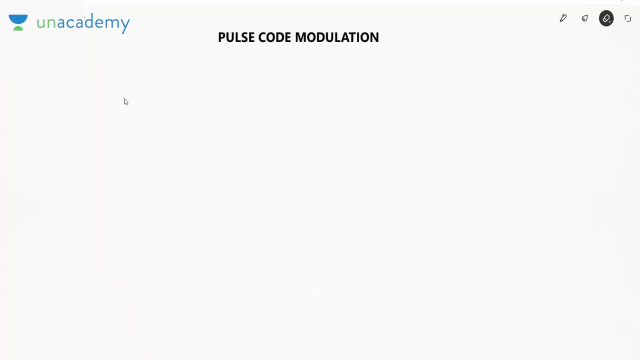 there will also be Hello friends, welcome to this lecture of communication system. So the last class we discussed about the basics of the digital communication and in that we understood What is the baseband digital communication and what is the bandpass digital communication. 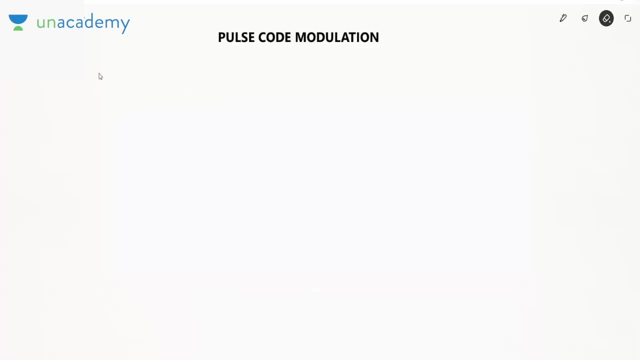 So in this class we will study another baseband digital communication technique, which is known as PCM. So first of all, the PCM is Baseband digital modulation technique. Now let me give you a brief idea about this PCM. so in case of PCM we take an analog. 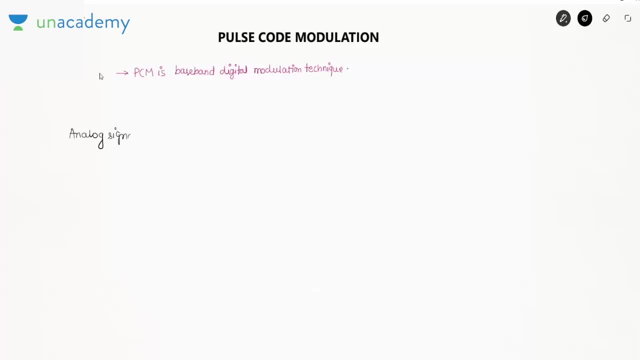 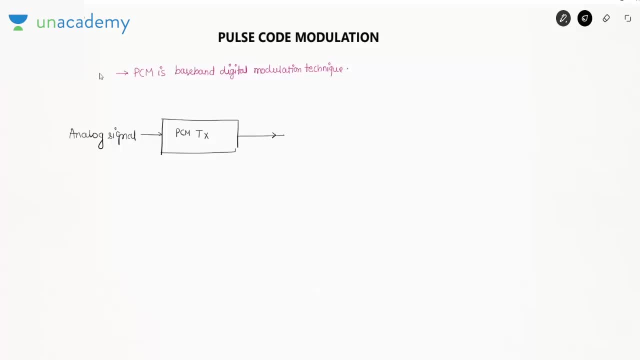 It is a signal. It is a signal. It is a signal. PCM is transmitted through the PCM Transmitter. PCM transmitter converts this analog signal into binary stream. After that, those binary streams are converted into different voltage pulses depending upon the number of bits being combined. 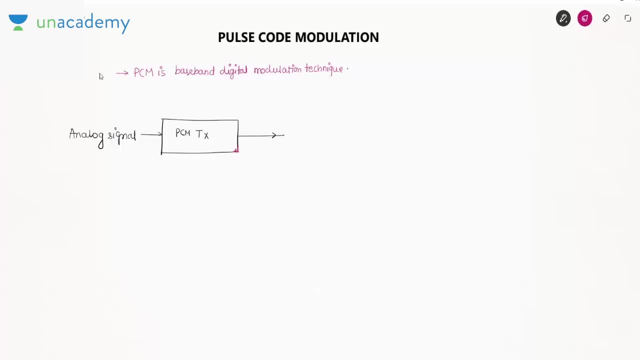 So we can combine one bit at a time, two bit at a time, three bit at a time, And so on, And based upon that we generate some voltage pulses out of those voltage pulses. One voltage pulse is transmitted at a time. 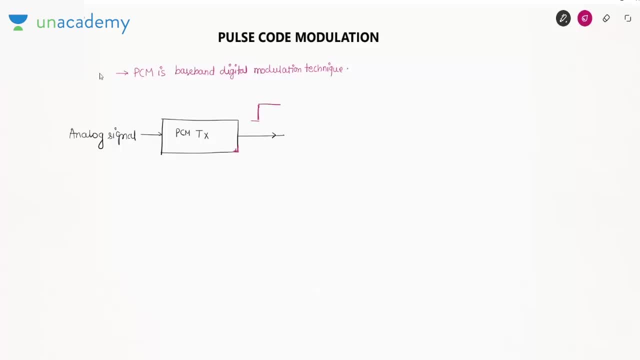 a time. so let us consider that at this time this voltage pulse is being transmitted. so we know that the nature of this voltage pulse is baseband, because in frequency domain it will be having nature of sync function, which is a baseband signal. so this signal is baseband signal. now, 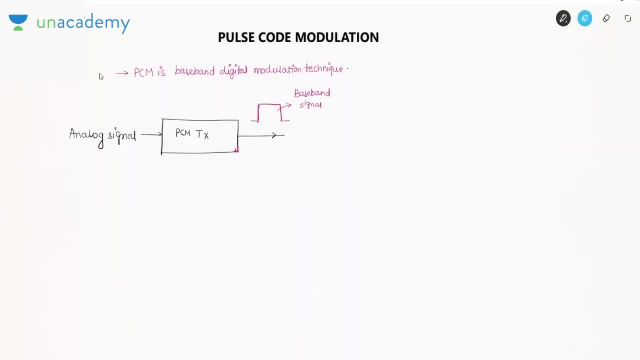 the signal is transmitted through the channel, since it is baseband signal, so it will be transmitted through a wire channel and somewhere in the wire the noise will get added to it. so let me call this baseband pulse as s of t, so the receiver will receive s of t. 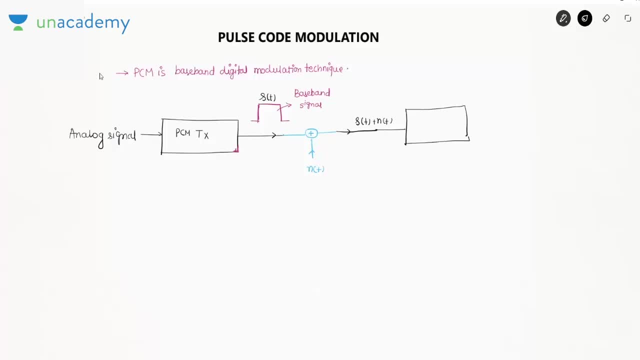 plus n of t, and here we will have pcm receiver. the purpose of the pcm receiver is to extract this analog signal from the digital signal and this extracted signal might have some error, so it can be the analog signal with some error. so this is the basic idea behind the. 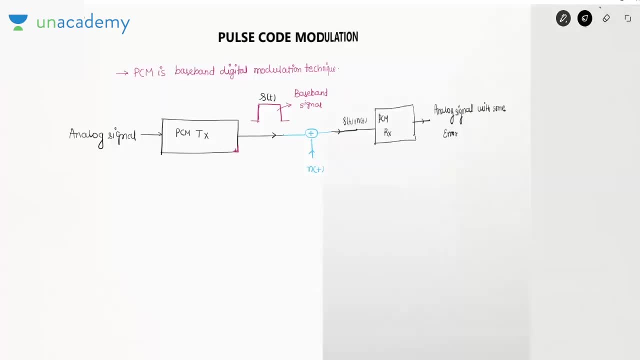 pcm transmission and reception. so now let us try to understand first of all the pcm transmitter or pcm modulator. so first of all i will draw the block diagram. after that we will try to understand each and every block in this diagram. so first of all let me start with analog signal. 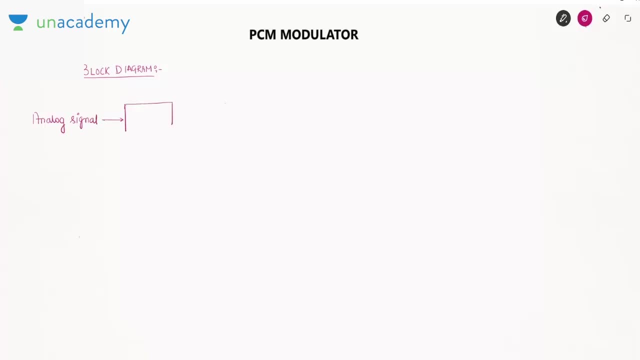 so this analog signal is: first of all is passed through an nt aliasing filter. let me call this analog signal as x of t. after that it is passed through a sampler, so it will have some carrier pulse strain which will help the sampler to perform the sampling. so 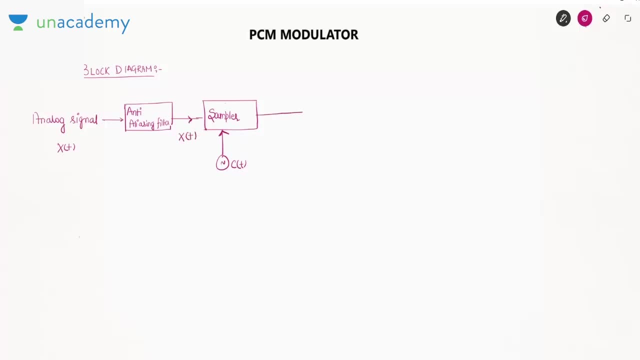 let me call this as x of t, and the output of this sampler will obviously be x of n, ts. now the output of the sampler is now fed to a quantizer. we know that a quantizer is defined with respect to its thresholds, so let me define its threshold. 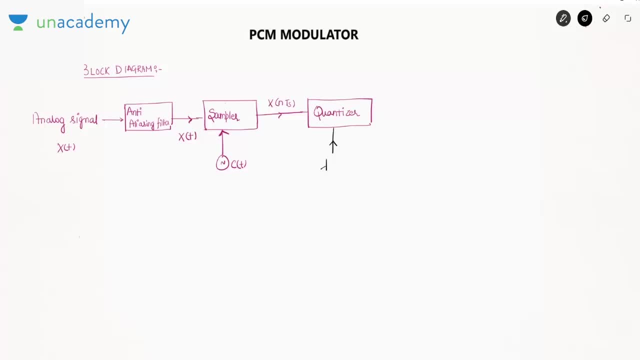 so what this quantizer will do? it will map the infinite number of samples to some finite number of quantization levels. so each sample which will be coming to the quantizer will be mapped to some predefined level. now let me define the output of the quantizer as: 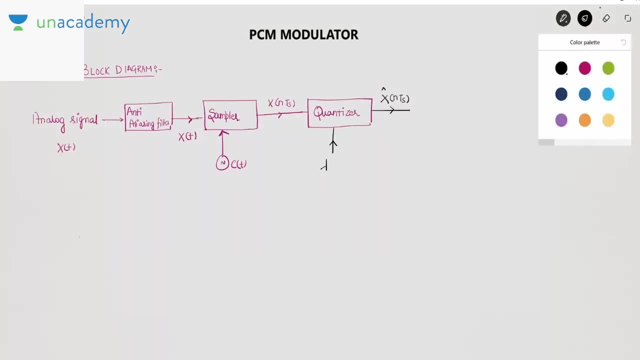 x cap nts. now, after the quantizer, we will place an encoder. so we will place an encoder here. the purpose of the encoder is to assign a unique binary code to each quantization levels. so here i am using this n, so it will assign n bit code word. 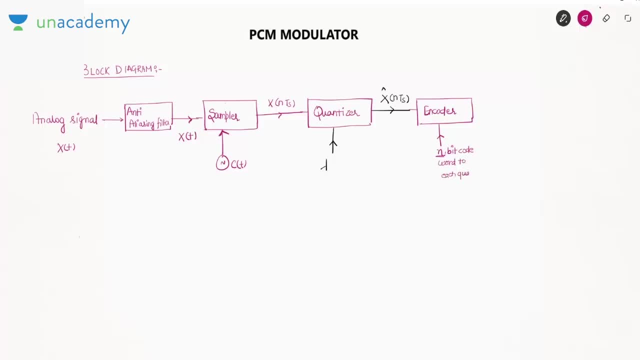 to each quantization level. now the output of the quantizer will obviously have. this output will have l levels and this encoder will assign a unique binary code to each level. then the output of the encoder is not Solved. then the output of the encoder is not Solved. 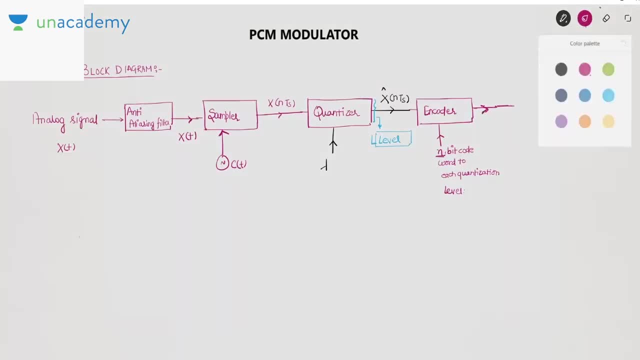 then the output of the encoder is not Solved. the encoder is now received by the line coder, so it is received by the line coder. so the output of the encoder is nothing but binary stream. so the line coder what will do? it will club the number of bits in the binary stream and 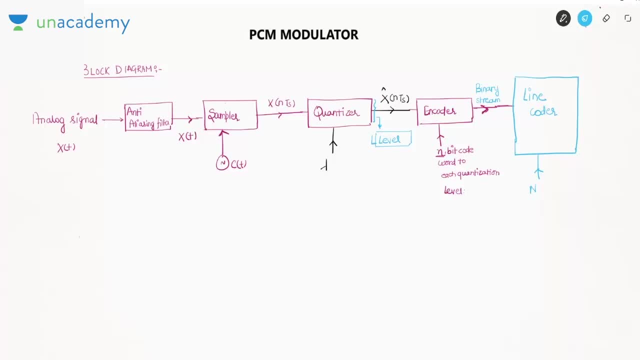 it will assign the voltage level to it. so basically, this line coder will convert this binary stream into a voltage waveform. so the output of the line coder is a voltage waveform or a waveform of voltage pulses. now, since each pulse will be baseband in nature, so after that a wire will be connected, or a channeled, or 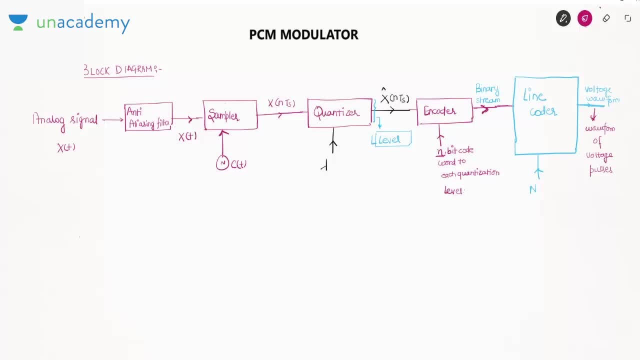 a wired channel will be connected so that these pulses will be transmitted by pulse, by pulse transmission technique. so now we will see how to convert this into a program. so let's, first of all we will. so now we will see how to convert this into a program. so let's first of all we 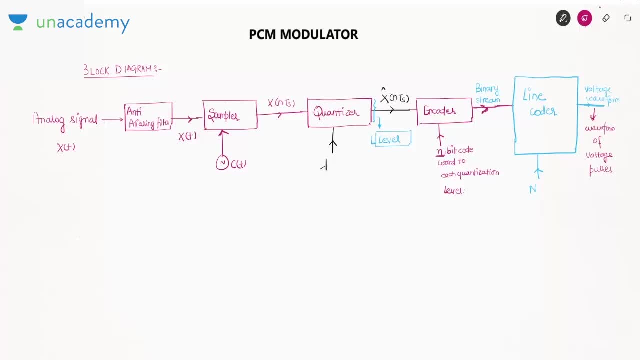 So now it will receive to the receiver. So this is the basic block diagram of analog signal. Now let us try to understand each and every component in it. So first of all, this analog signal is x of t. it is being passed through the anti aliasing. 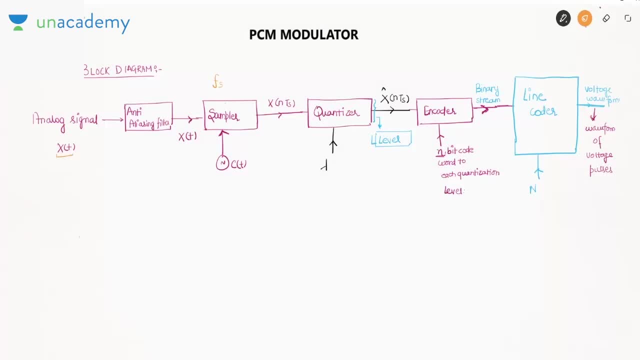 filter. We know that we can reconstruct our message signal from the sample signal only when fs is greater than 2 times of fmax. So this is the restriction on the sampler. Now suppose our x of t is having infinite bandwidth, or it has the maximum frequency. 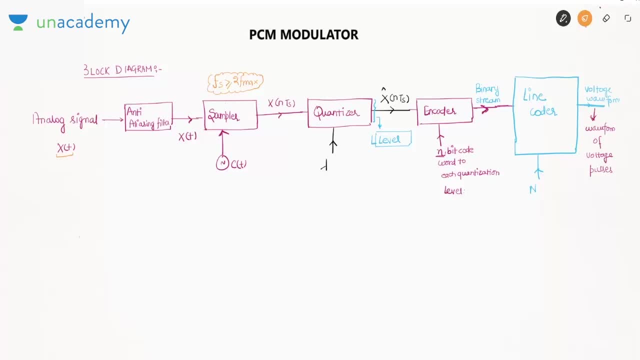 component as infinite. So we can never find a sampling rate which by which the sampling should be performed so that the sample signal could be recovered. So, as a precautionary measure, any incoming signal, first of all, is band limited to some finite frequency by this anti aliasing filter. 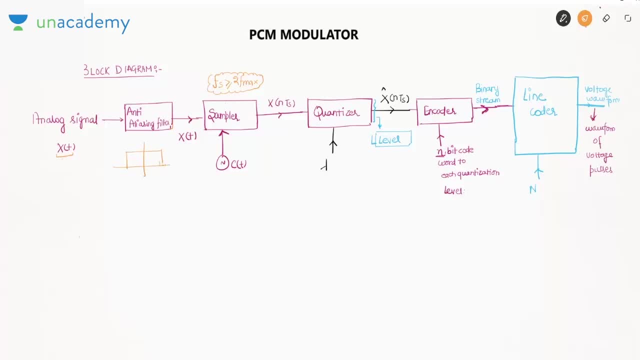 So this anti aliasing filter is nothing but a low pass filter and generally it is band limited to some fs by 2.. So any incoming signal which is having infinite bandwidth should be band limited to some fs by 2, and then the sampler will always have a sampling. 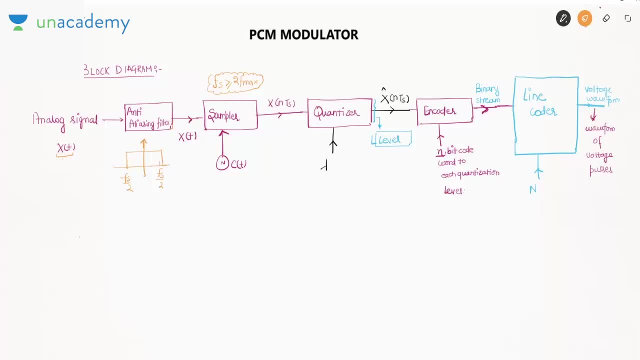 rate by which it should be sampled, so that the sample signal can be reconstructed into its original message signal. After that, this x of t is passed through the sampler, so sampling will perform its sampling, and if fs is greater than 2fmax, so the sample signal can also be reconstructed back. 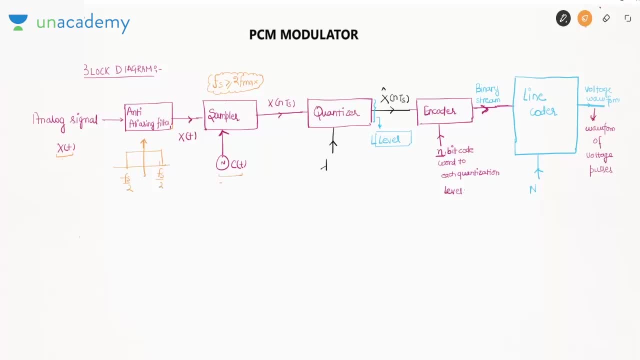 Now for sampling any signal, we need the impulse train or any carrier train. so this is representing your carrier train Now. after that, this sample signal is passed through the quantizer. so, based upon the decision levels or threshold levels, the quantizer will divide its dynamic range into different, different. 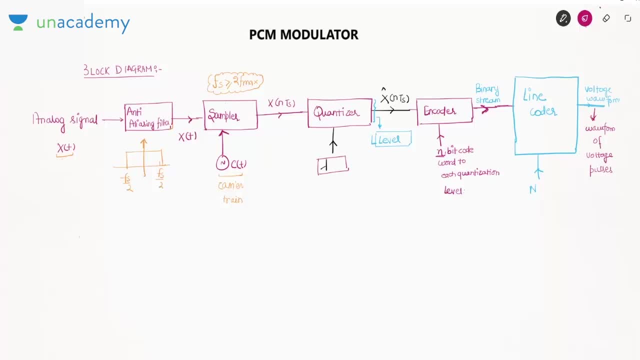 regions, and each range will be mapped to a predefined level, So the output of the quantizer will have L levels. Now the encoder will assign a unique binary code to each quantization level or each level, So that Each sample which is coming from the sampler will have a binary code. 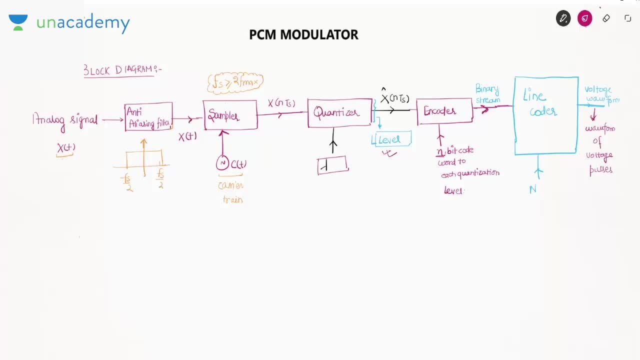 So after that the encoder output will be converted into a binary stream. Now line encoder will pick either 1 bit at a time, 2 bit at a time, 3 bit at a time and so on, and based upon that it will generate a voltage, pulses and then pulse by pulse transmission. 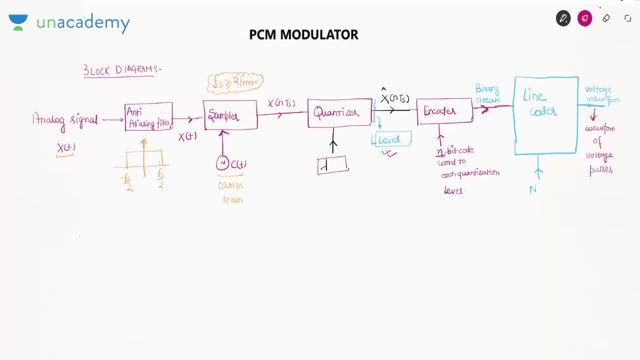 is taking place and since each pulse represents a baseband signal, so we use the wired transmission of these pulses. So this is the basic idea behind the PCM modulator. So, first of all, the first block which you are seeing here is NT aliasing filter. 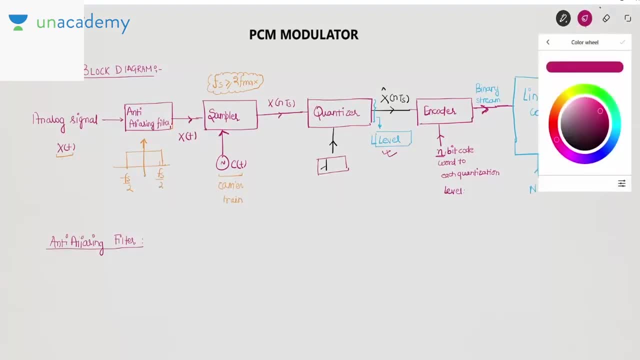 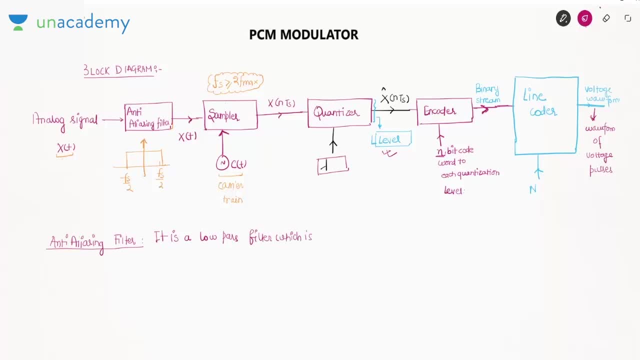 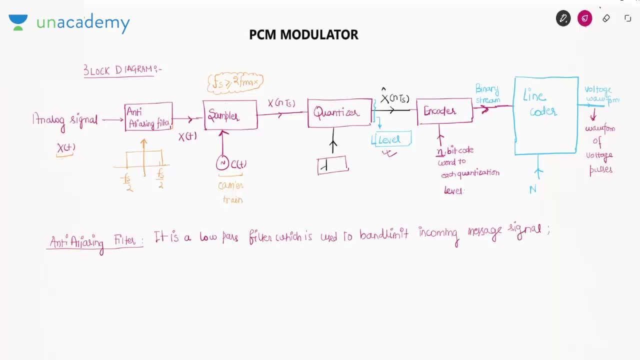 signal so that signal is transmitted via honeycomb. So now Sampler can have finite sampling rate. for sampling Generally the cutoff frequency of anti-aliasing filter is equal to fs by 2. So it is generally half of the frequency of the sampling rate. 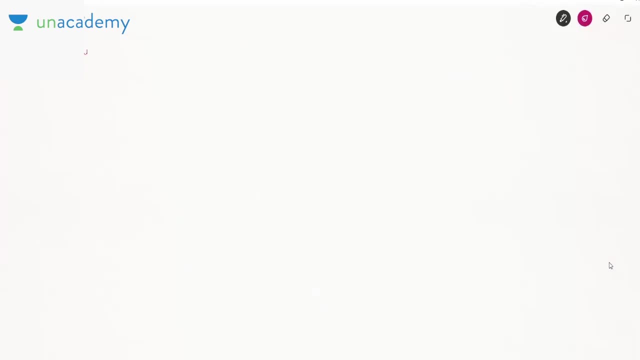 Next block is sampler. We know that sampler will convert x of t into x of nts and you can reconstruct back from x of nts to your x of t Only when fs is greater than or equal to 2 times of fmax. 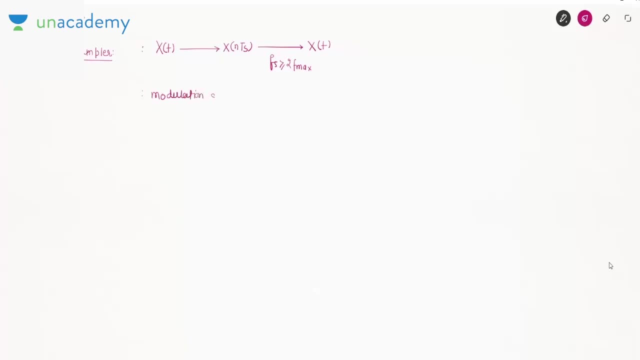 Sampling is also a modulation scheme in which characteristics of carrier pulse strain. Carrier pulse strain is varied in accordance with: In accordance with baseband message signal. In accordance with baseband message signal. So it also represents some sort of modulation. Now, after the sampler, we will have a quantizer. 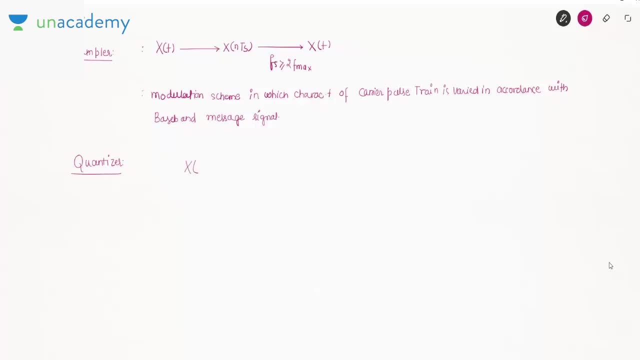 We know that quantizer will have sampled signal as input and this is the quantizer. so the output of the quantizer will be x cap of NTS. This will be Lambda. So first of all, This Lambda will divide the dynamic range of quantizer. 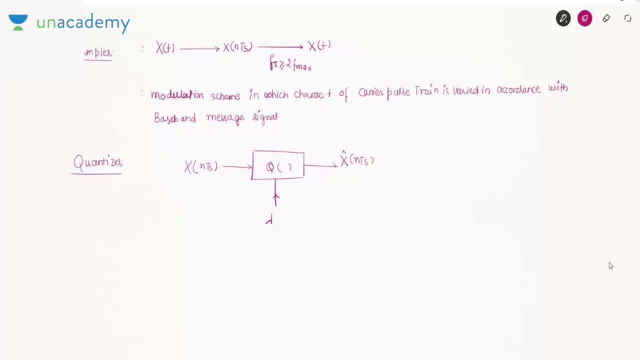 NTS will be lambda into different different regions and generally the dynamic range of the quantizer matches with the dynamic range of incoming signal so that each region of the dynamic range can be mapped onto the single value by the quantizer. so the output of this quantizer is quantized. 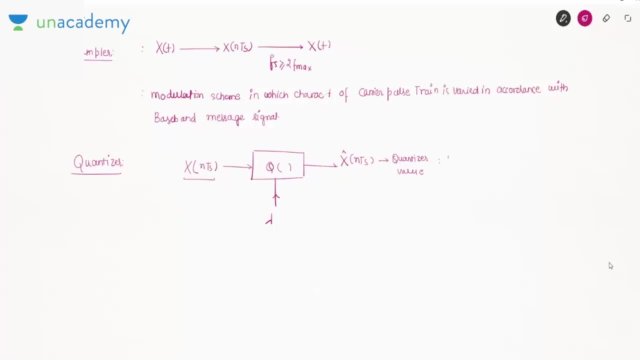 value and this output will be divided into L quantization levels. so, based upon this decision thresholds, the dynamic range will be divided into different different regions and each region will be mapped onto a single value and, basically, at the output of the quantizer is called as quantized value and it will have total L different quantization levels. now 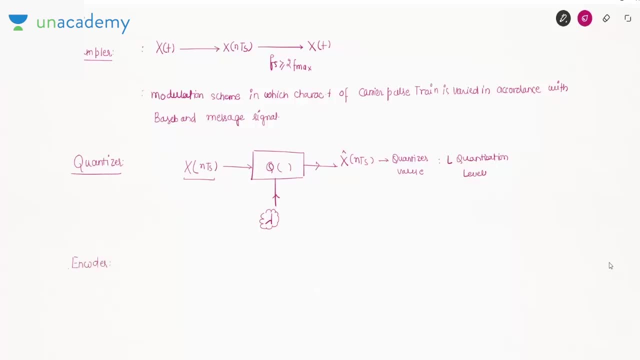 So next block here is encoder. so, as we said, that encoder assigns unique binary code to each quantization levels, quantization levels. so we can define small n, which is number of bits assigned to quantization level. now we know that whenever the quantizer will receive a sample signal, so first of all it will quantize it to any one of the levels. 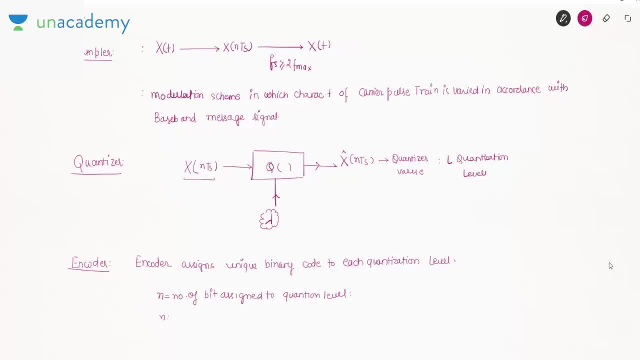 and then encoder will assign it a binary code. So small n can sometimes also be defined as number of bits per quantized sample. so the sample signal will reach at the input of the quantizer. the quantizer will map it to any one of the quantization levels and the binary code assigned to that quantization level will. 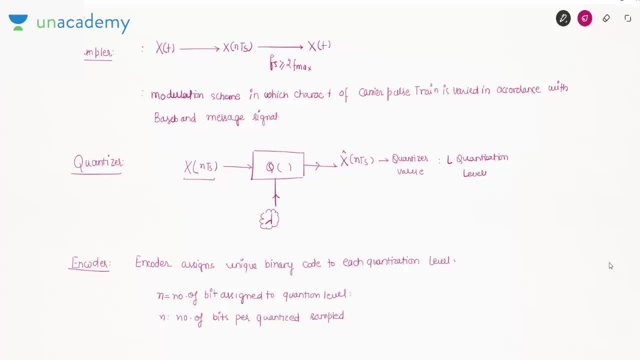 be assigned to that quantized sample. So in this way each quantized sample will be given an n-bit binary code. So each quantized sample will be given to given n-bit binary code. after the encoder we will have linecoder. 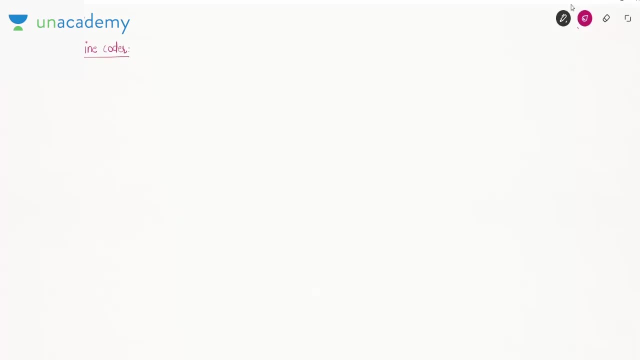 The purpose of the linecoder has already been explained in the last class. but again, the linecoder will Give, As will combine bits in binary stream and each combination of bit, each combination of bits, is assigned a voltage level. so the output of the line coder will be output of line coder. 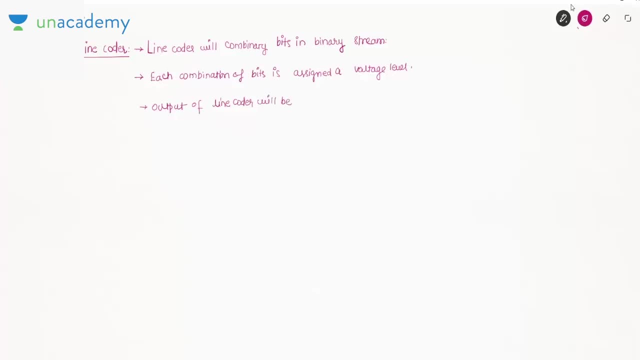 will be a waveform of a of voltage pulses. so the output of the line coder will be waveform of voltage pulses. now, each voltage pulse, each voltage pulse represents a baseband, a baseband pulse or signal. so pulse by pulse transmission, pulse by pulse transmission, takes place via wired channel. 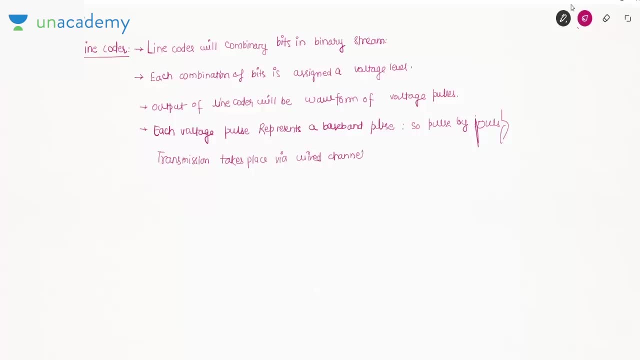 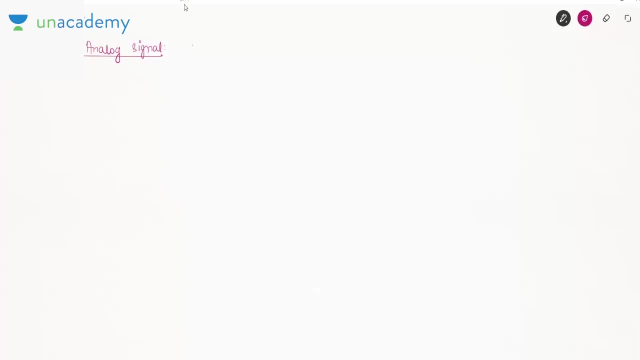 so now let us try to understand it by an example. so this is your analog signal, раж signal, This is your X of T. This is zero. Let me call this instant as TS, This instant as 2 TS. This is 3 TS. 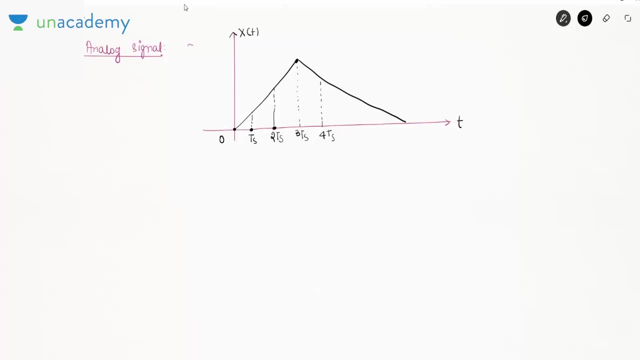 Again, this as 4 TS, This point as 5 TS And this point as 6 TS. So this is the analog signal And these are the sampling instances which are represented here. So let me call this value as 1.. This value as 2.. 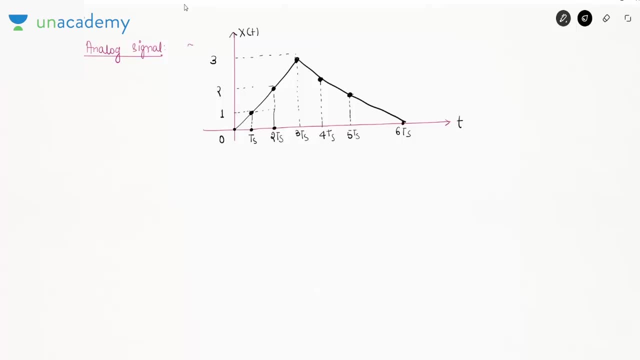 This value as 3.. So these values will be same here. Now, what will be the sampled output? So the output of the sampler or the sampled output? So the sampled output will be X of NTS. So it will be sampled like this: 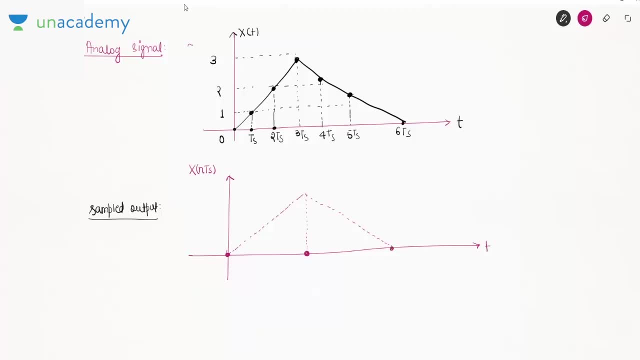 So this frequency or this instance will become zero And the sample at this instance will be zero. This point will become TS And this amplitude will become 1.. So this is the sampled output. At 2 TS It will have sampled value of: 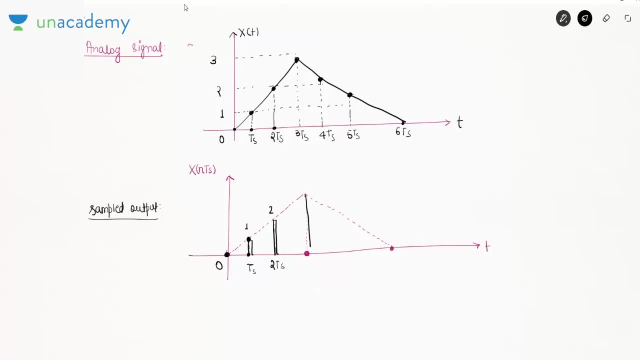 2.. At 3 TS, We will have sampled value of 3.. Again at 4 TS, We will have sampled value of 2.. Again at 5 TS, We will have sampled value of 1.. And at 6 TS, 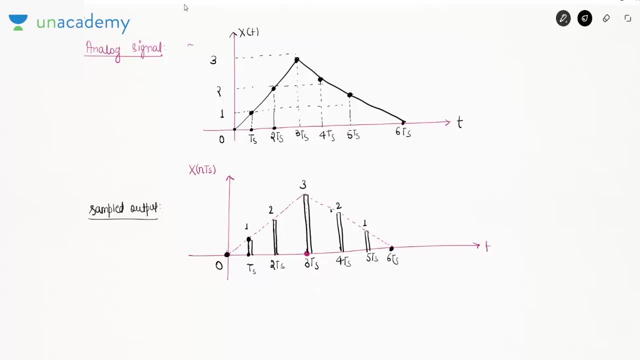 We will have sampled value of 2.. We will have sampled value of 0. So this is our sampled signal. Now, this sampled signal has dynamic range from 0 to 3.. So this is the dynamic range, which is from 0 to 3.. 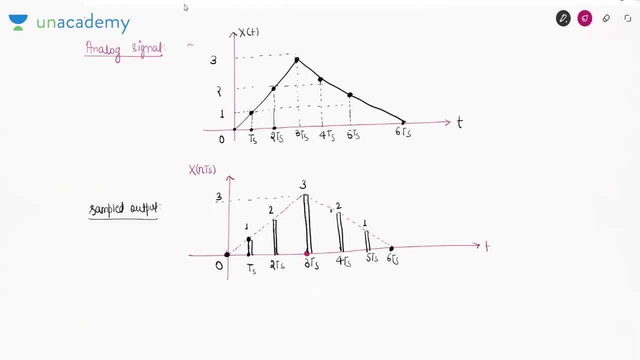 Now it is being passed through the quantizer. So this is the sampled signal X of NTS And it is being passed through a quantizer And the output of the quantizer will be X cap NTS, And here I am defining lambda as 1.5.. 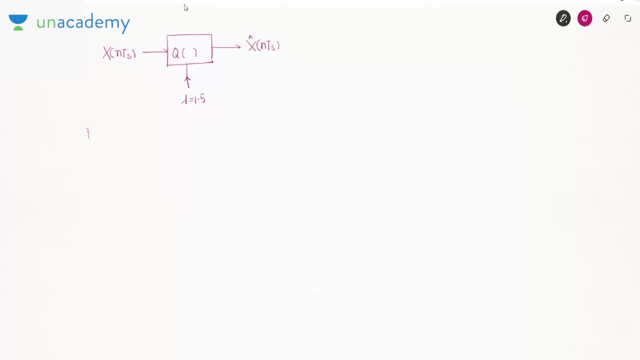 So first of all I am considering that dynamic range of X of NTS and dynamic range of quantizer matches. It may or may not match, But here I am assuming that it is matching the dynamic range of the quantizer. So first of all let us consider that at the quantizer input, at the quantizer input, this: 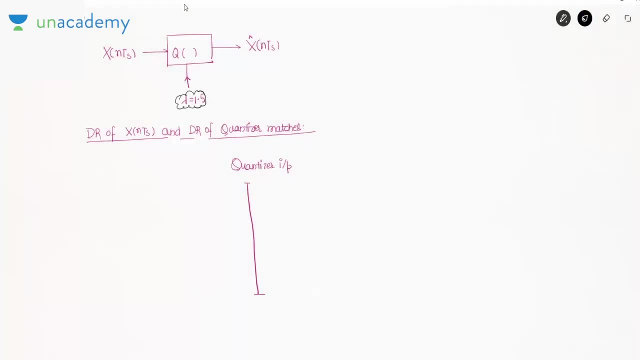 threshold, which is lambda equal to 1.5, will divide the quantizer dynamic range into different different regions. So this is your lambda equal to 1.5.. And the quantizers dynamic range varies from 0 to 3.. So we are assuming that if this is our x of NTS, 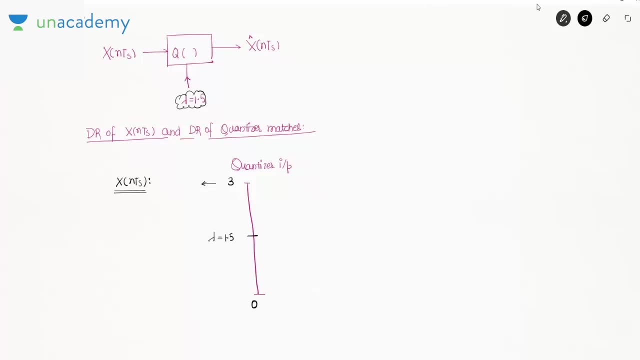 So the dynamic range of X of NTS exactly matches with the quantizer. So the quantizers dynamic range is varying from 0 to 3 and this will match with this X max And this will match with this X min of the signal. So here the dynamic range of the x of nts, which is from x min to x max. 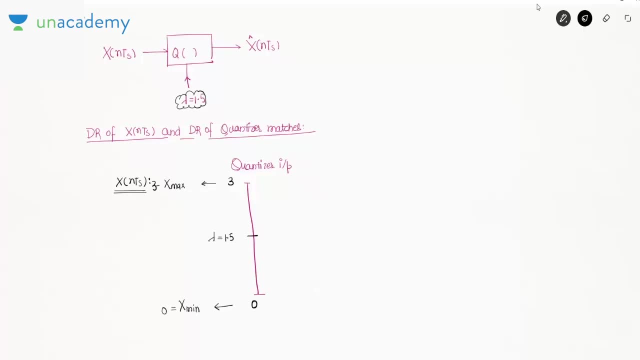 or from zero to three, is matching to the dynamic range of the quantizer, And here we have taken the threshold level 1.5.. So it will divide the dynamic range of the quantizer into two different parts. So what will be present at quantizer output? So the range of values which 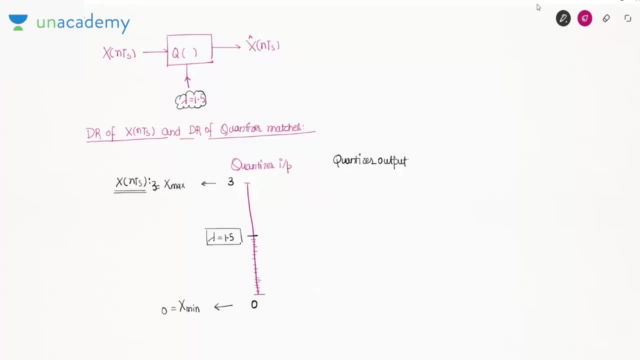 is coming from zero to 1.5. these all will be mapped onto a single quantization level or a single value, which is 0.75.. Similarly, all the voltage levels which is coming from 1.5 to 3 is being mapped to 2.25.. So we can say that this quantizer is mapping all the 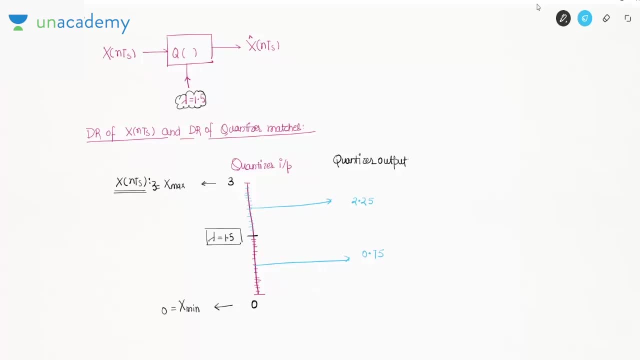 incoming signal into two different levels. So we can say that it is having two level quantizer, or we can say that each incoming signal is being quantized into two levels. Now here you have to understand the working of the encoder, what encoder basically does. so encoder will observe the quantizer output. 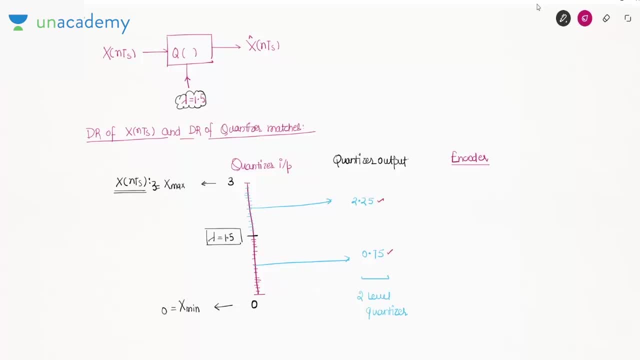 it observed that quantizer has only two different outputs, 0.75 and 2.25, so it has basically two different outputs and it has to assign a unique binary code to each quantized output. so you can see that, since it is having only two quantized output, so it can use only one. 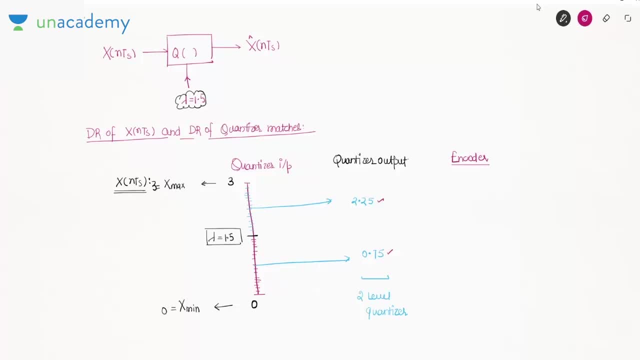 bit binary code for each of the quantization levels. so it may assign it bit 0 and it may assert this level as one. so what is the meaning of that level as 0? or this level is 1? you can very clearly see from this that the input of the quant consol is the value that varies. 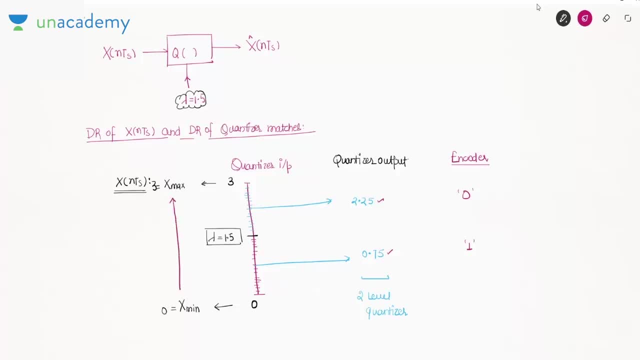 from 0 to 3, so this quantizer can have any value between 0 to 3 and the quantizer will map any value of zero to three in any one of these fourputters, cdc of any value of 0 to 3 in any one of these fourpisa. 3 or bc of in any of these fourputters. 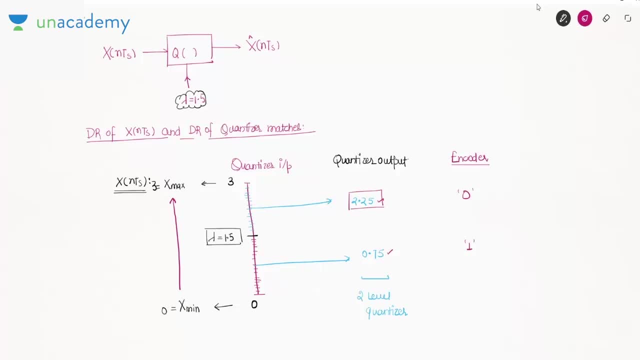 these two quantized levels. so it may map it to 2.25 or it may map it to 0.75. so each incoming signal will be either mapped to 2.5 or 0.75, or we can say that whenever any signal is. 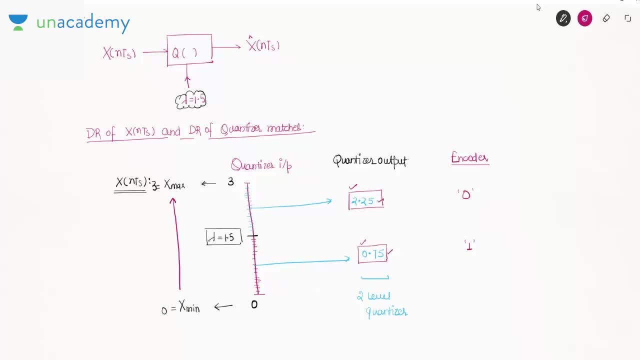 incoming to the quantizer input, it will map it to 0.75 or 2.25. if it is being mapped to 0.75, the encoder will assign it a binary code of 1, and if the sample value is being quantized to 2.25, the encoder will assign it a 1 bit binary code, which is 0. so we can also say: 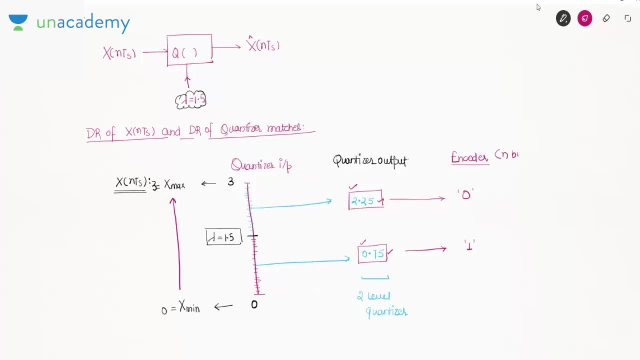 that the encoder will assign n bits per sample, so we should more clearly write it as n bits per quantized sample, but in general you can also say that it is assigning n bits per sample. each sample which is coming having the value of 0 to 3 will be quantized to these two levels. 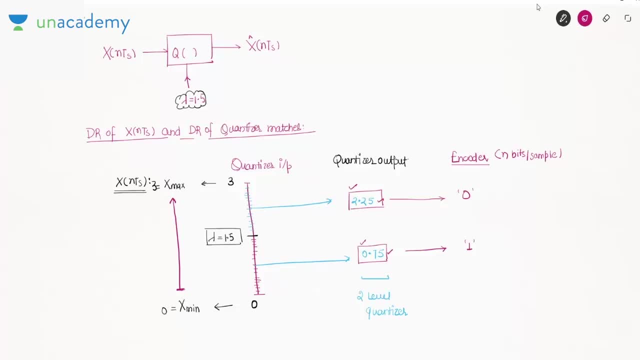 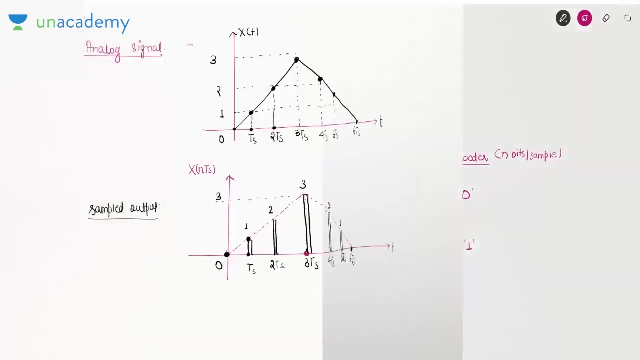 only, and the encoder will assign that sample a particular n bit, which is in this case 1. so this is the operation of this encoder. now let us try to understand what will happen here. so this was the sampled output. now the output of the encoder will be 0.25. so this: 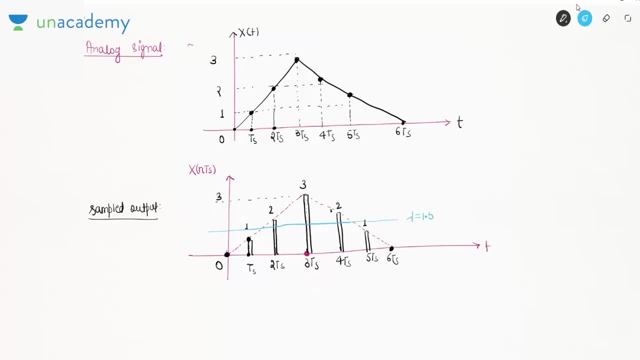 is the output of the encoder. this is the output of the quantizer, output which will be based upon the value of lambda. so the all the sample values which are below this will be mapped to 0.75 and above this will be mapped to 2.25. so the output of the quantizer will. 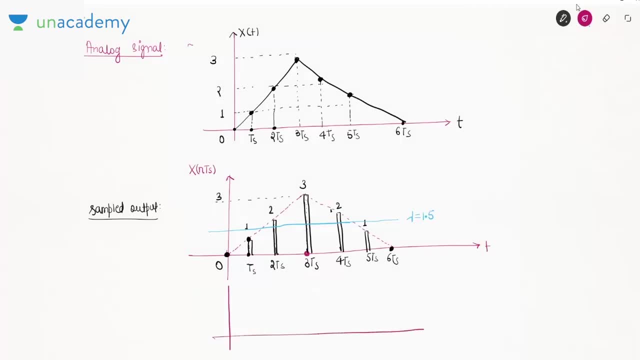 look something like this: so this is the quantizer output. so how the quantizer output will look like, let us try to understand. so this sample value 0- it is also below 1.5, so it will be mapped to 0.75 at 0. at TS, this sample value is 1, so it will be also mapped to 0.75. this. 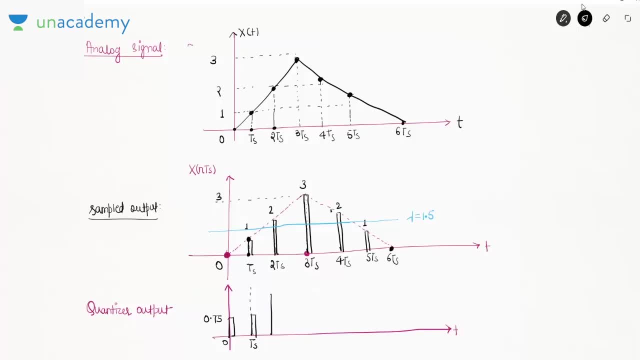 value is above 0.125, so it will be mapped to 2.25. similarly, at this point, this value will also be mapped to 2.25. at 4 TS, this value will also be mapped to 2.25, and these two values will again be mapped to 0.75. so this value is 2.25 and all these values which are 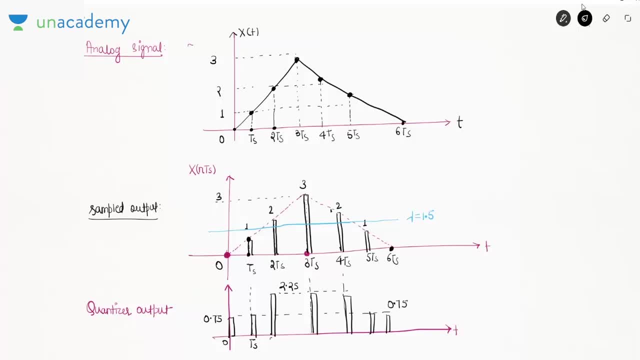 here are at 0.75 and obviously this time instances are TS, 2 TS, 3 TS, 4 TS, 5 TS and 6 TS. so these are the quantities, Quantizer output, or the graph of X, cap and TS. so now let me draw this diagram again. so 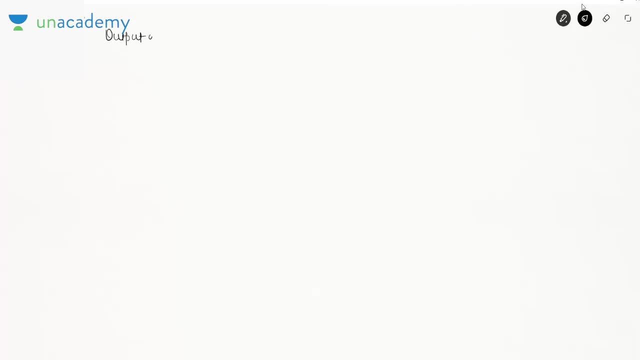 the output of the quantizer that we have obtained here was something like this Quantizer output, or the graph of X, cap and TS. this is NTS, so here we will have 0.75 at 0, then also at TS, then at 2 TS, at 3 TS, at 4 TS, 5 TS and 6 TS. so this was as 2 TS, 3 TS, 4. 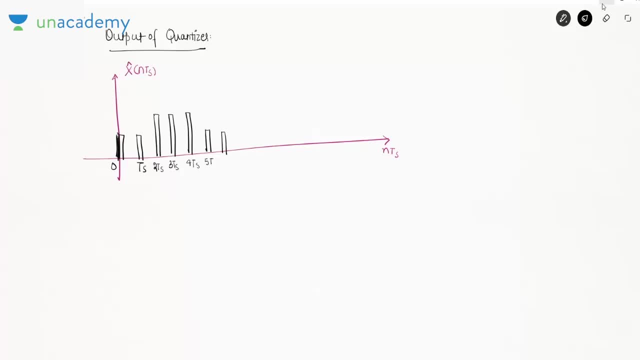 TS, 4 TS, 5 TS and 6 TS. so these values are at 0.75 and these values are at 2.25. now what encoder will do? encoder will assign a unique binary code to each quantized value. so the encoder will assign bit 0 to all the samples which are being mapped to 0.75, and it will 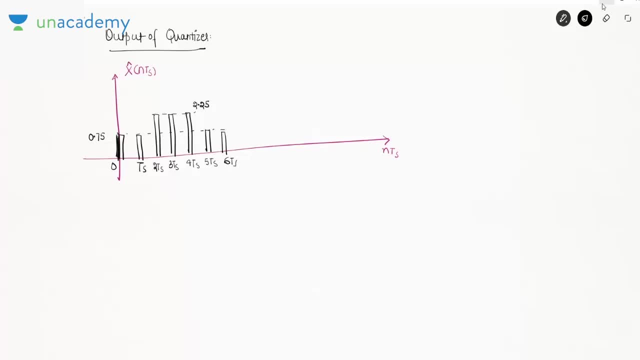 assign: 1. 1., 1., 1., 1., 1., 2., 2., 1., 2., 2., 4., 4., 5., 6., 7., 6.. 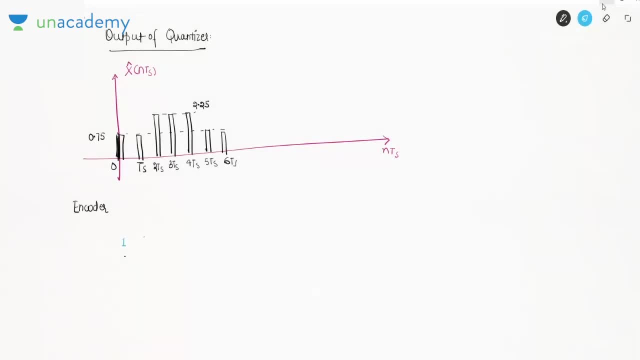 7., 8., 9., 10., 11., 12., 13., 14., 15., 16., 17., 18., 19., 20. 21.. assigned binary 0, and which are being mapped to 0.75, has been assigned to binary 1.. 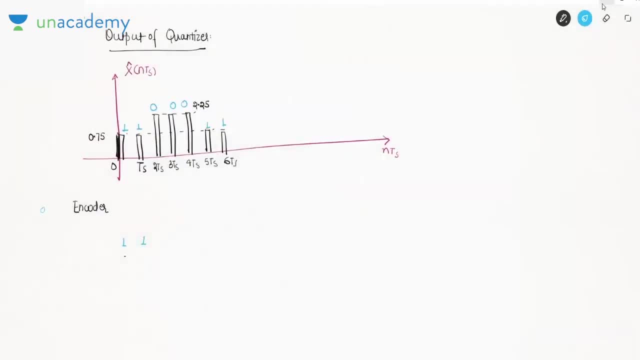 So, similarly, the output of the encoder will be 1100011. or you can say that the output of the encoder will be a binary stream, So this is the binary stream. Now this output of encoder is fed to linecoder. So this is our linecoder. 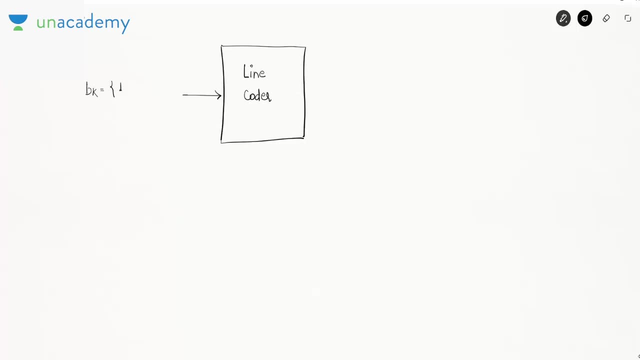 So this is bk equal to 1100011.. Let us assume in this case we are clubbing one bit at a time and, based upon that, we are generating a voltage waveform. So what it is doing, it will club one bit at a time and it will generate a voltage pulse. 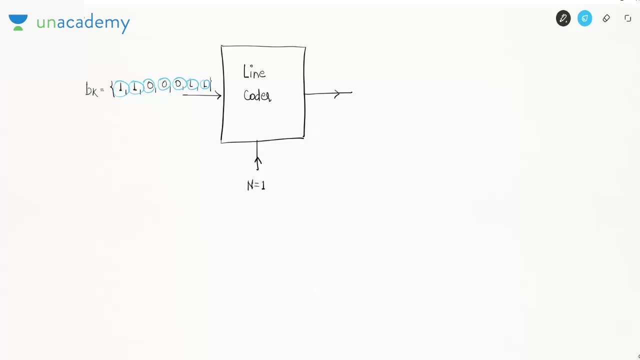 accordingly. So first of all, it will club bit by bit. And let us assume that for bit 1, it is generating a voltage pulse of amplitude A and duration TB, And for 0, it is generating a voltage pulse of amplitude minus A and duration TB. 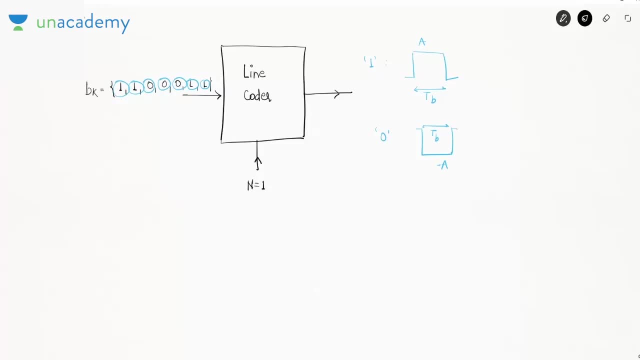 So here what we are doing for representing this 1 and 0, we are using the rectangular shaping. Or we are representing bit and 1,, 1 and 0 by rectangular pulses. So we are using this rectangular shaping. You can also represent this 1 by a sinc pulse in time domain and a negative sinc pulse in. 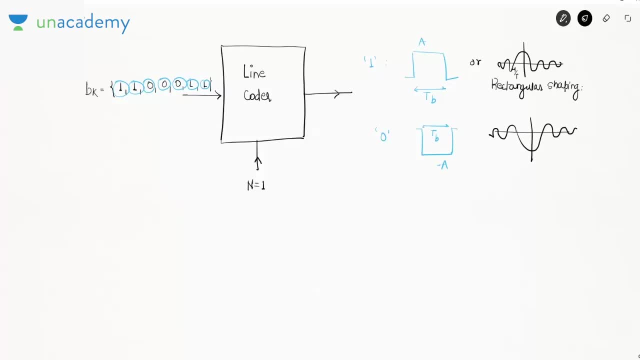 time domain. So this will be minus 1 by TB. So this will be negative sinc pulse in time domain And this point will be 1 by TB. Similarly, here also, this point will be 1 by TB And this point will become minus 1 by TB. 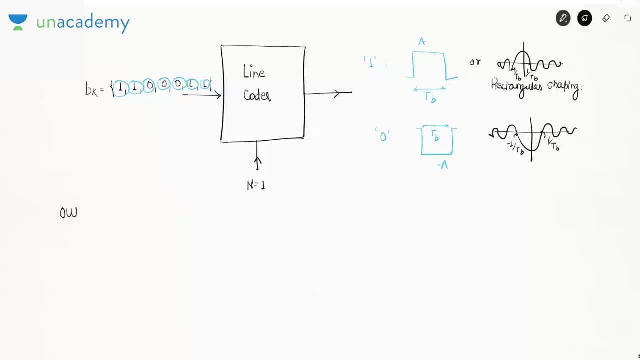 So now let us try to represent the output of line coder. So the output of the line coder might look like this: This was the binary stream. it will assign a voltage level of A to 1,, then again 1, then it will assign a voltage level of 0, then again 0,, then again 0, then it will assign. 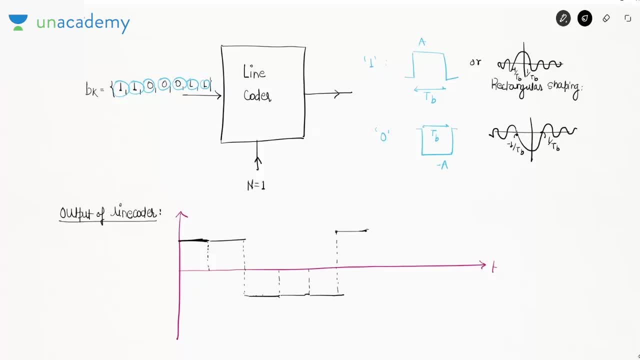 a voltage level of 1 and 1.. So this will be the binary stream. This will be the voltage waveform which will be present at the output of the line coder if rectangular shaping has been used. So this will be A. this duration will become TB. this will be 2 TB, 3 TB, 4, TB, 5, TB, 6. 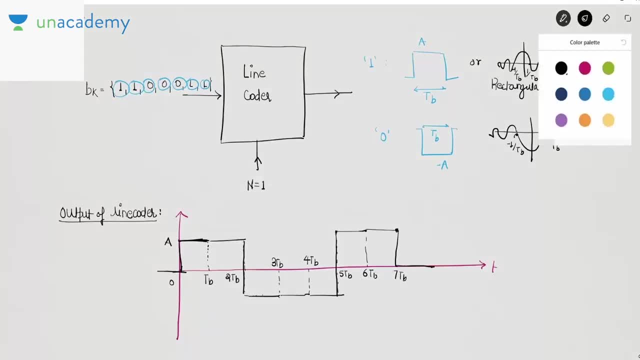 TB, 7 TB and so on. It will represent bit 1, bit 1, 0, 0, 0.. Bit 1 and bit 1.. Now, after that, what will happen? this particular waveform which we are receiving here is known. 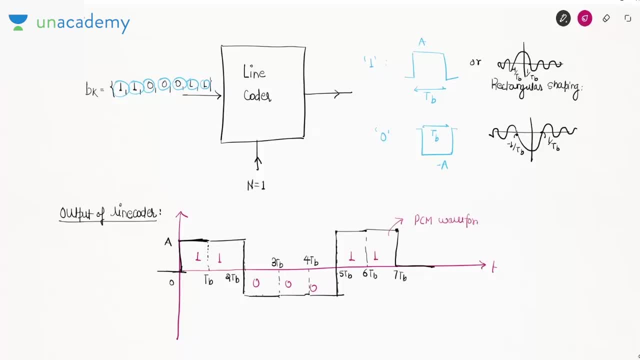 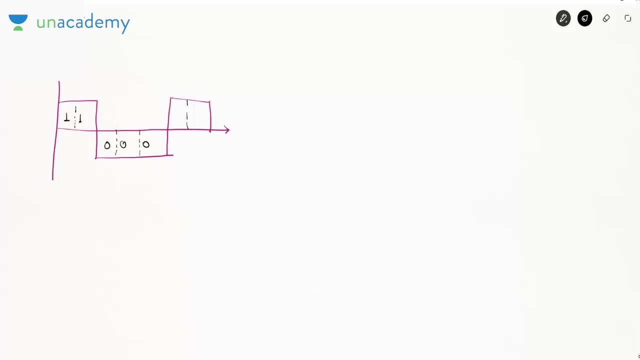 as PCM waveform. So this PCM waveform will now be transmitted through a wired channel. So this PCM waveform which we generated here, So the PCM waveform which we generated here- 1, 1, 0, 0, 0, 1, 1,. the duration of each pulses: 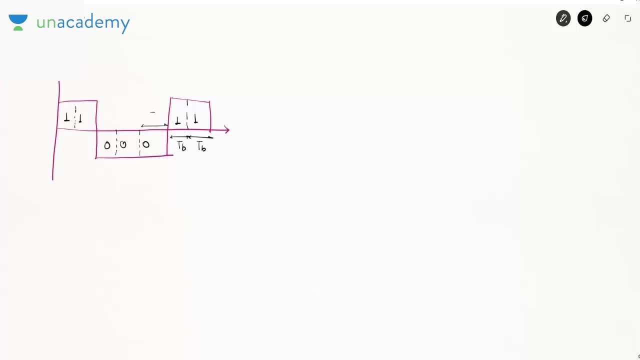 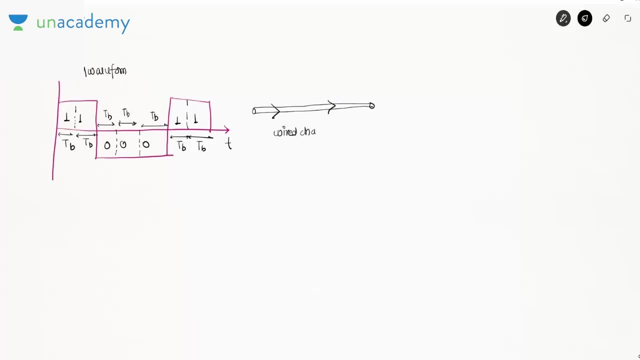 So it is transmitted through a wired channel. Now, at a time, through the wired channel, pulse-by-pulse transmission will take place. So pulse-by Pulse transmission, Pulse-by-pulse transmission will take place. middle long, Middle long. 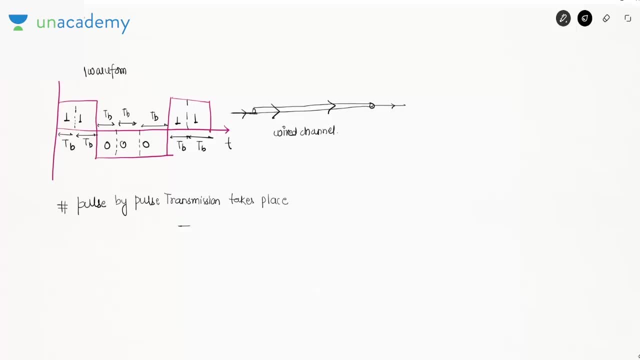 Middle, Middle long, Middle long, Middle long through wired channel, which means at a time, only one pulse will be transmitted through the channel. So this will be the scenario: that this pulse will be transmitted at a time through the channel. We know that after the band limiting the frequency spectrum can. 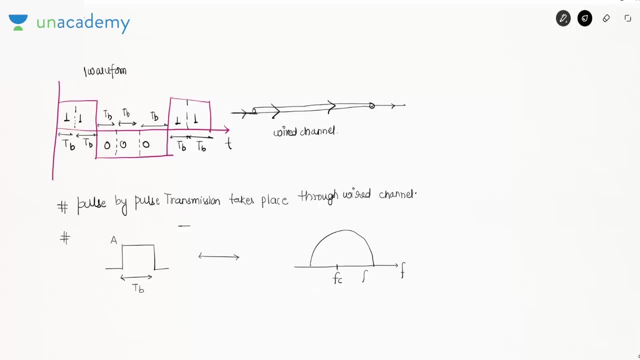 be drawn something like this, So it will become Fc. This is Fc plus 1 by Tb. Fc minus 1 by Tb. sorry, So this will be 0,. it will be 1 by Tb. it will be minus 1 by Tb. 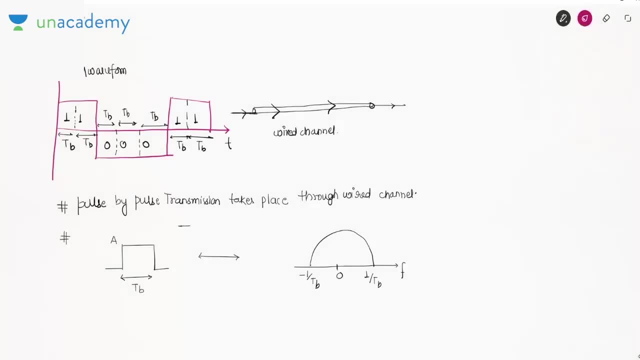 So bandwidth of this pulse is from 0 to 1 by Tb. or you can say that bandwidth of one single pulse is 1 by Tb when rectangular pulse shaping has been used, or it is equal to 1 by Tb. So the wired channel should have bandwidth which should be greater than or equal to 1. 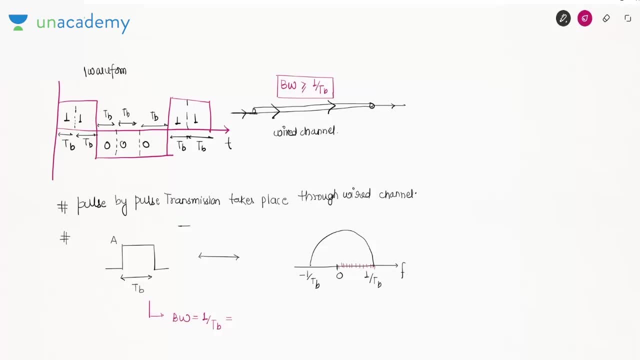 by Tb. So the bandwidth of the wired channel when PCM waveform is non-linear transmitted should be greater than or equal to 1 by TB when rectangular pulse shaping has been used. now let us try to understand what happens if we have used sink shaping. so for sink, one sink pulse will be transmitted at a time. so this: 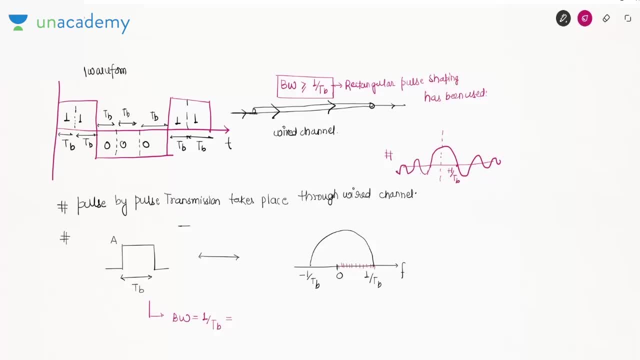 point is minus 1 by TB. sorry, 1 by TB. this point is minus 1 by TB, and this is T. we know that the frequency spectrum of the sink pulse will be a rectangular pulse in frequency domain, so this will be a rectangular pulse in frequency domain. so this will be a. 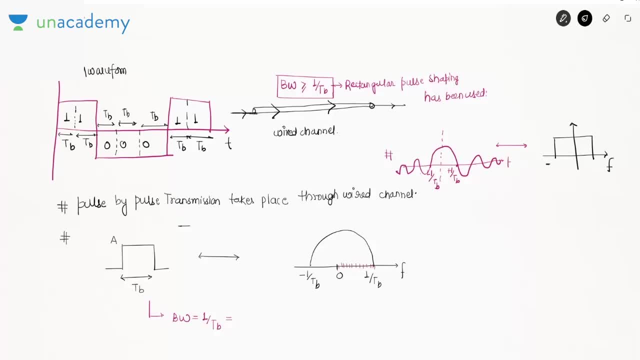 T, this will be F and this will be minus 1 by 2 TB to 1 by 2 TB. so the bandwidth of for each pulse comes out to be one by 2 TB. so from here you can also say that since bandwidth of each pulse is 1 by 2 TB when a sink pulse shaping has been. 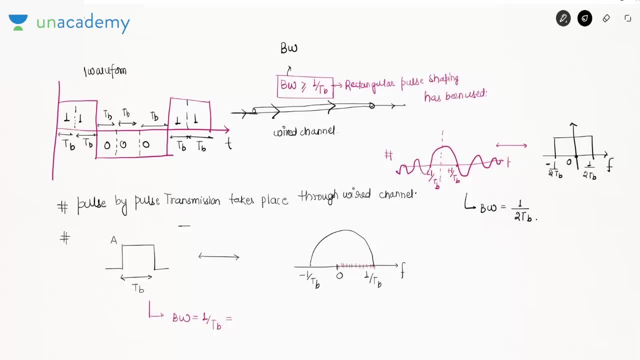 used. so the bandwidth of the wired channel should be either greater than or equal to 1 by 2 TB when sink pulse shaping, sink pulse shaping has been used. So since pulse by pulse transmission is taking place if the shape of the pulse is rectangular, 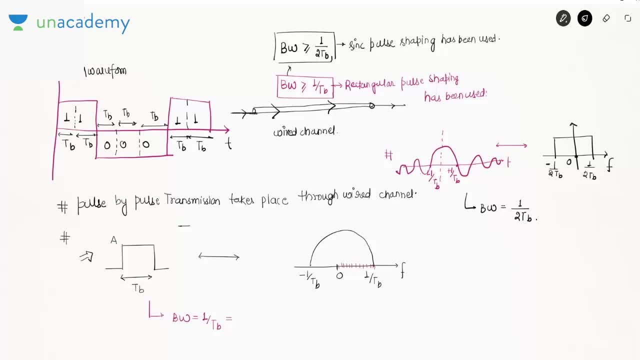 then the bandwidth should be greater than or equal to 1 by 2 TB. sorry, 1 by TB, because the bandwidth of each pulse is 1 by TB- and obviously the channel bandwidth should be greater than the bandwidth of the pulse. and if sink pulse shaping has been used, then 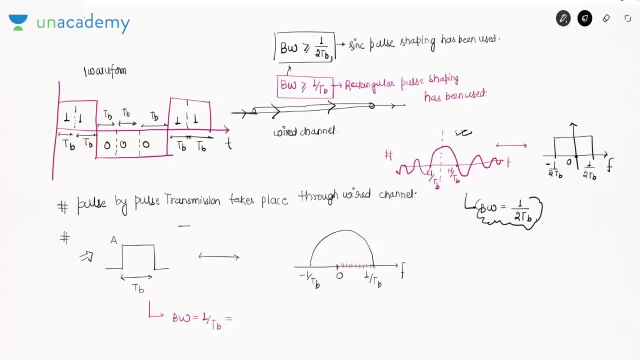 the sink pulse shape will have bandwidth of 1 by 2 TB. So in this particular case, the bandwidth should be greater than or equal to 1 by 2 TB when sink pulse shaping has been used, because the channel bandwidth should always be greater. 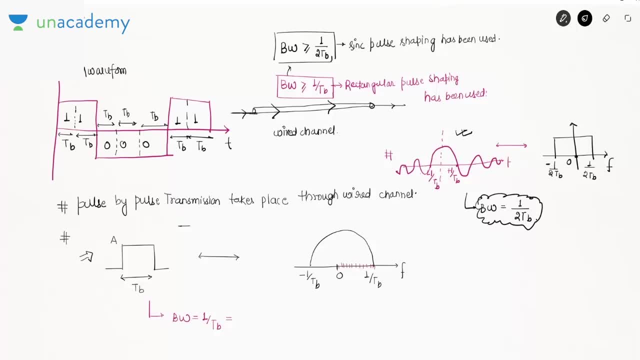 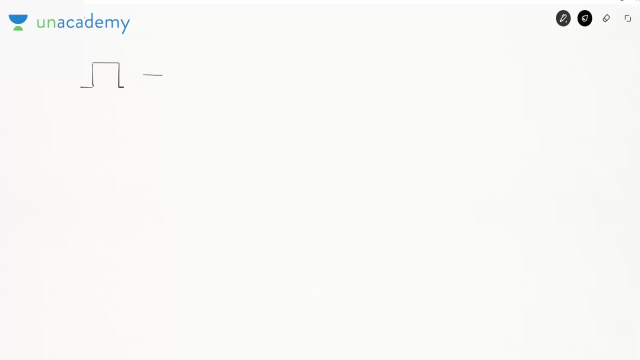 than the bandwidth of the transmission. Now these pulses travel through the wired channel, So this is the wired channel and somewhere in the wired channel the noise gets added. So suppose I'm calling this voltage waveform as ST and the signal which will be receiving. 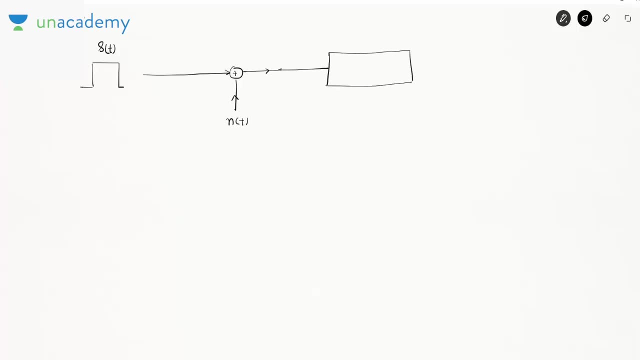 to the PCM receiver is ST The pulse plus the added noise. the noise has been added in the channel. So now, after that, let us try to understand how the PCM receiver extracts the analog message signal from this transmitted voltage pulses through the wired channel. 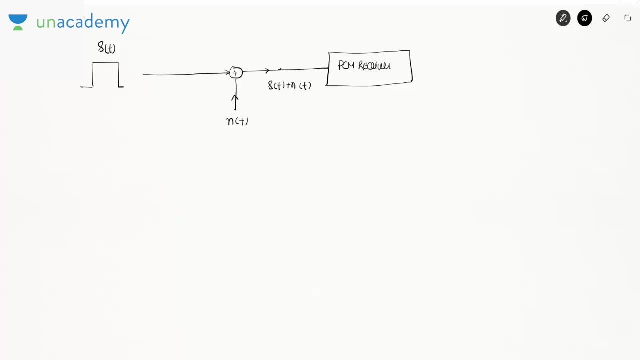 So first of all let us try to draw the basic block diagram of the PCM receiver. Then afterwards Let us try to understand each and every block of it. So the PCM receiver will look something like this: So this is the PCM demodulator or PCM receiver. 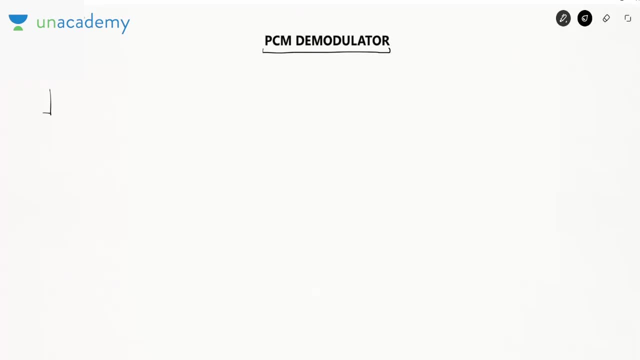 So the input of the PCM will be this: pulse S of T plus channel noise. So first of all we will have block of regeneration circuit. So this circuit is known as regeneration circuit. It contains decision making circuit. Okay, Okay, Okay. 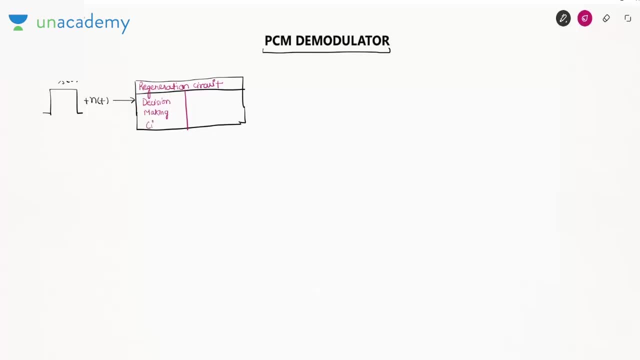 Okay, decision making circuit and pulse generating circuit. So basically it filters out the noise and it tries to regenerate this signal or the pulse s of t again. So each incoming pulse is passed through it. So it processes the noise, or it removes the noise and tries to 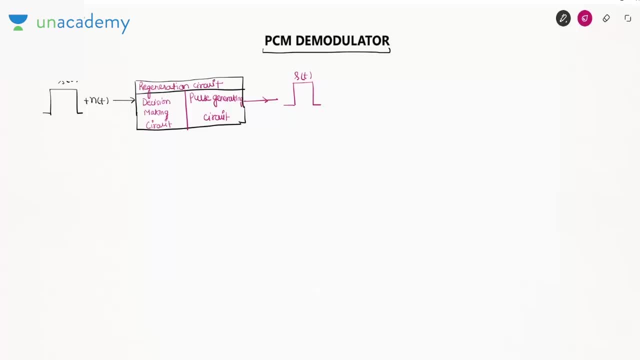 regenerate the same signal back. Sometimes it can, sometimes it does not. This gives the rise of the problem of the probability of error. So if this decision making circuit and pulse generating circuit is able to extract exactly the same signal being transmitted, then there is no 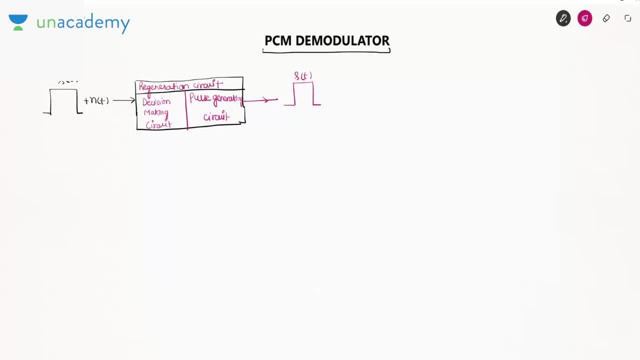 probability of error. And if they are not able to extract the same pulse, then there may be probability of error or error might occur. Then this pulse is passed through a decoder which is acting inversely as of encoder, So the encoder's input will be decoder's output and 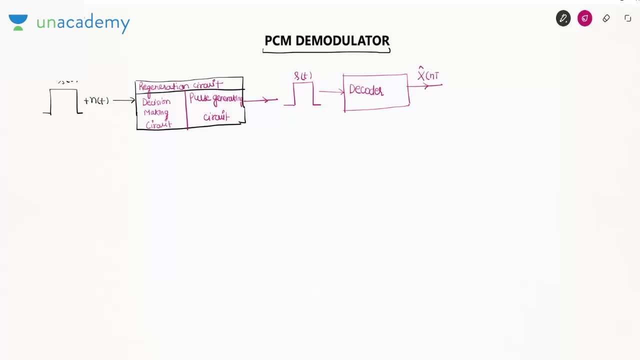 encoder's input was quantized signal. So here we will get again back x, cap and ts. Then we will use a reconstruction filter. So here we will use a reconstruction filter, which is generally a low pass filter, And then the output of this reconstruction filter will be an analog signal and 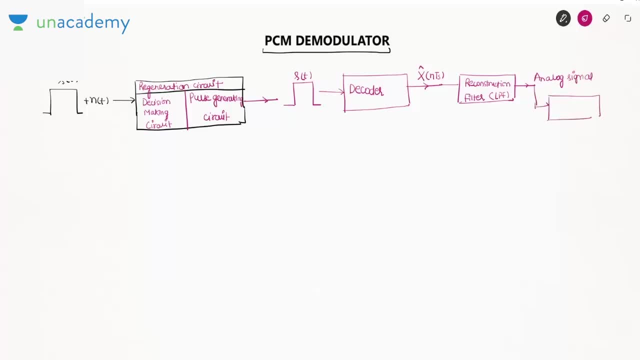 this signal must be transmitted to the destination. So this is the block diagram of PCM receiver. So x, cap and ts is the output of decoder at the receiver. Now this x, cap and ts block diagram is something like this. So this x cap and ts which has been 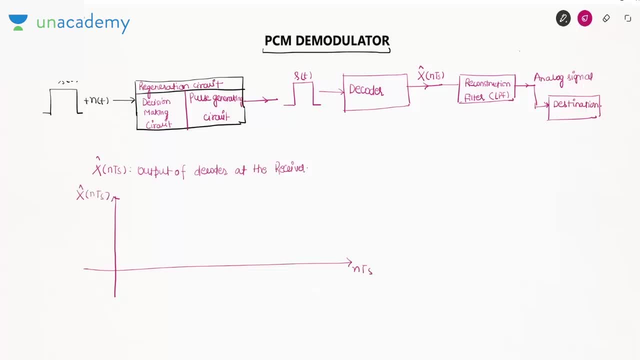 recovered at the receiver will look something like this: It is again the 0.75, 0.75,, 2.25, 2.25,, again 2.25.. Then 0.75 and 0.75.. This amplitude is 0 ts, 2 ts, 3 ts, 4 ts, 5 ts and 6 ts. All these amplitude. 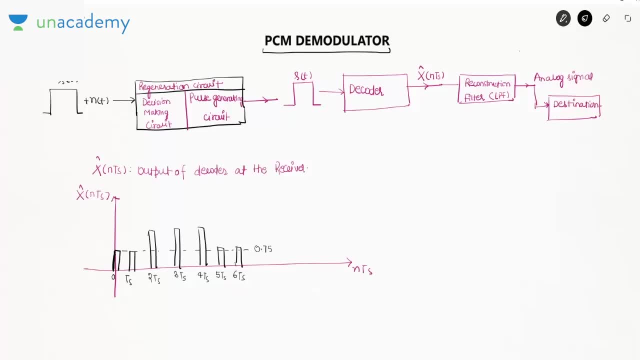 levels are 0.75.. And these amplitude levels are 2.25.. Now this signal is passed through a low pass filter And we have to observe the output of the low pass filter. So this output we need to observe. So this is the input to the low pass filter. So this is the input to the low 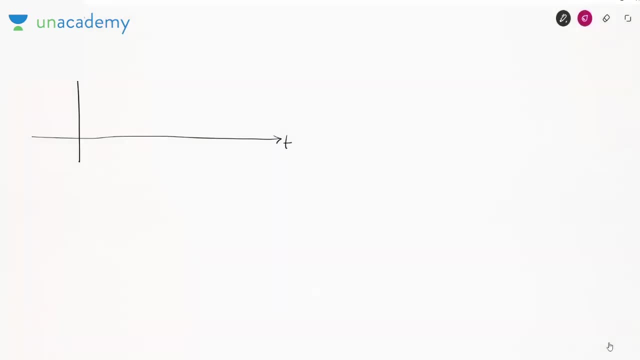 pass filter. Now we can plot the view with this value, So we can draw the value, value as it is. So this value will this value Then at the receiver 6 cap and 6uez. Then we will write together this value in this relation. 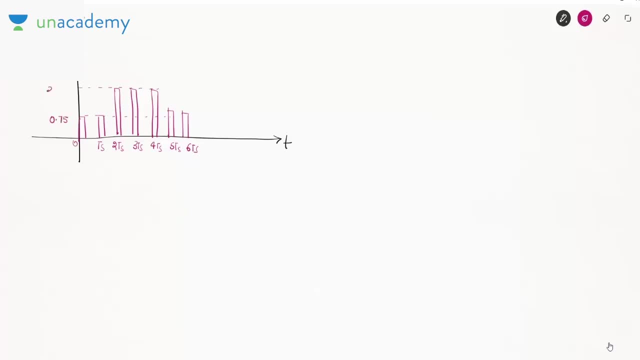 So I least say this, and it is this value equal to 0.75.. So this is the value to this value, and this value is equal to 0 to 151.. So this value is equal to 2.75.. However, this becomes two point two, five, and this is X cap NTS. so this is your low-pass filter. 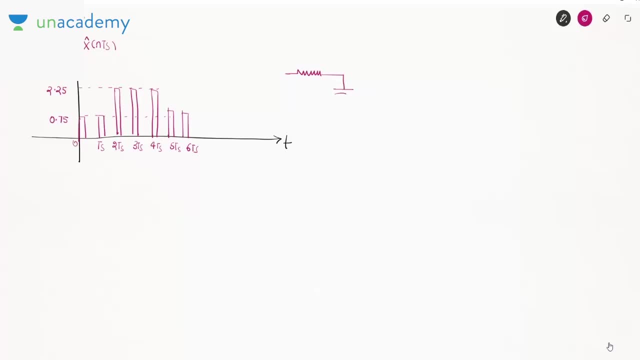 this is our C and we have to plot the output. so first of all, you should notice here that this low-pass filter I am considering here, first of all I will, I will draw the output for ideal low-pass filter, then we will try to connect it with practical low-pass filter. so this is the output. 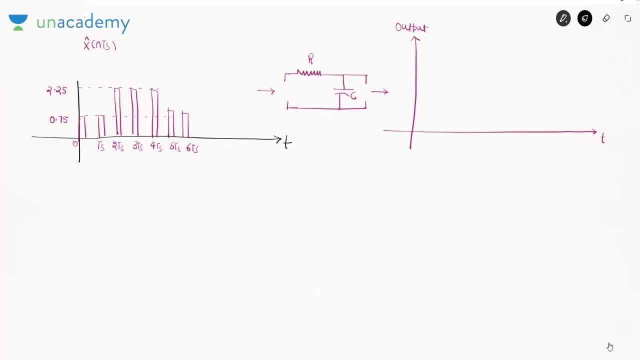 this is the T. so what will happen here? as soon as this 0.75 pulse comes at the input of this low-pass filter, this low-pass filter gets immediately charged to this value. so these are the input values of the low-pass filter. so 0 Ts, 2 Ts, 3 Ts, 4 Ts, 5 Ts, 6 Ts. so as soon as this voltage comes, 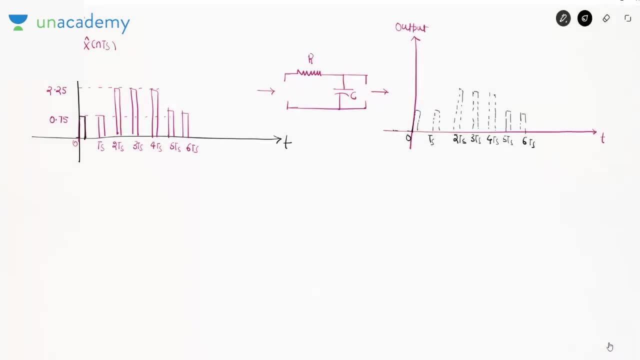 the output gets charged up to this value and it remains charged up to this value till the next voltage comes. so the next voltage is again 0.75, so it remains up to the 0.75. then, as soon as the voltage comes, which is at the level of 2.25, this capacitor gets charged to 2.25. 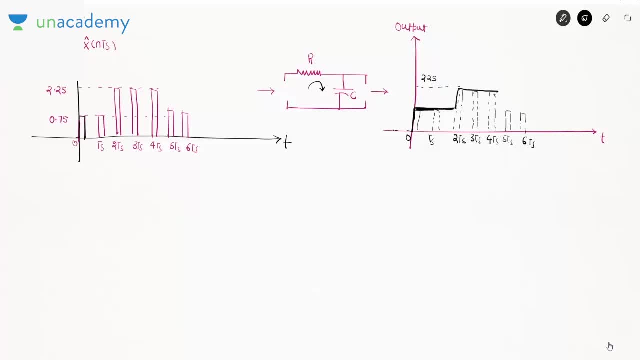 and it retains up to 2.25 because the voltage is not changing. at 5 Ts the voltage decreases to 0.75, so this capacitor also discharges to 0.75 and it remains at 0.75 at some instant. 7 Ts. 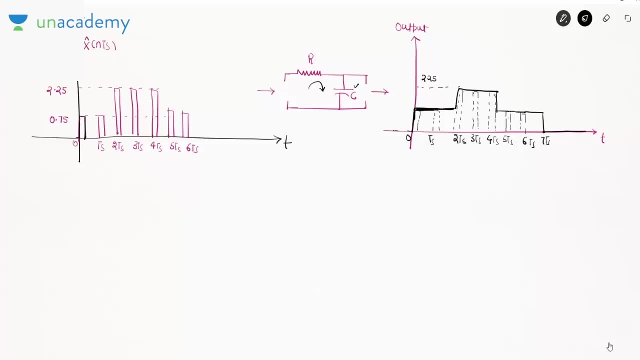 it gets discharged to 0 volt. so this is the output of the ideal low-pass filter. what will be the output of the practical low-pass filter in practical low-pass filter? this charging, discharging will be rather smooth, so it may look something like this now, if you notice, the transmitted signal was 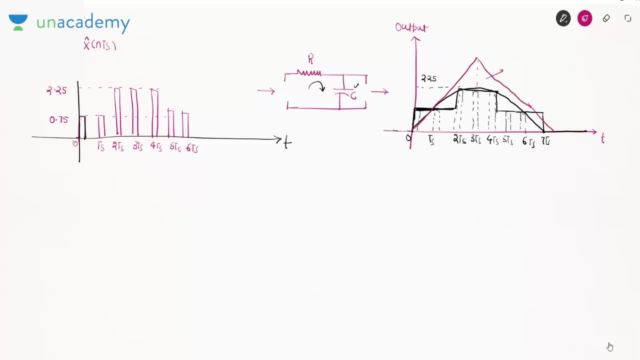 something like this: this was the transmitted analog signal and this was the received analog signal, and in between you can see that there is some kind of error and this error you can call it as quantization error. so this error where the quantized signal is not able to approximate the main signal. 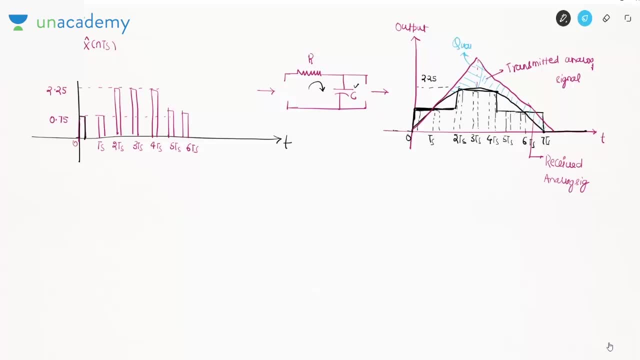 so this error is called as quantized error. so the recovered signal at the receiver will not be exactly equal to the transmitted analog signal, but it will have some error which is known as quantization error. and quantization error can never be removed. it will always be present in the recovered signal. so this was the idea behind the PCM. 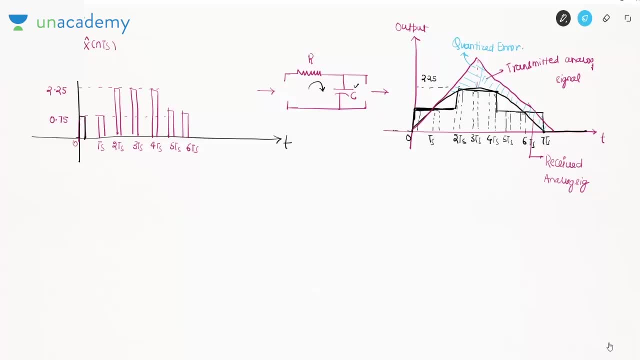 transmission and reception. in the next class we will try to understand few more terms related with the PCM. we will see the formulas of the PCM. so thank you. so hopefully we have understood every concept in this class. if you have any doubt in any concept, you can let me know in. 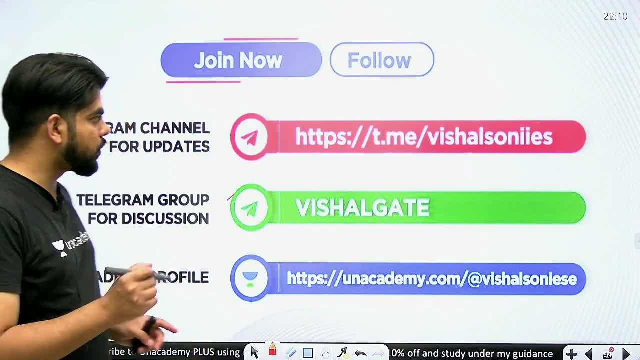 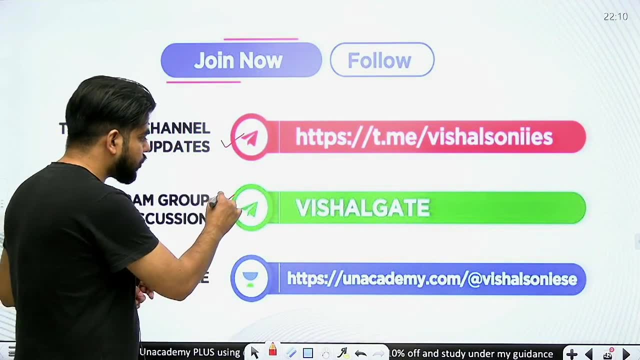 the comment section. I will try to resolve that thing. apart from that, you can also follow me on various social media platform. for example, you can join this telegram group where you will be getting important notification, important updates. this is telegram group where you can also commit, you can ask your queries or maybe you can also suggest me for the improvement. 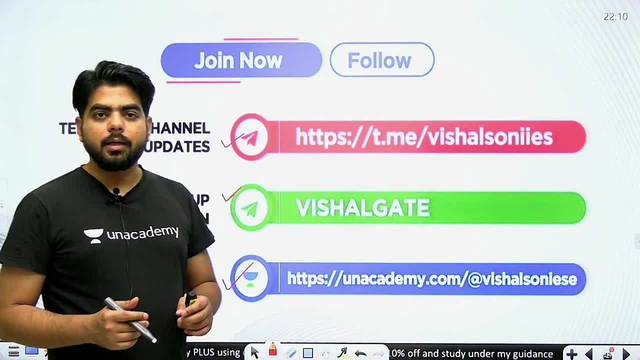 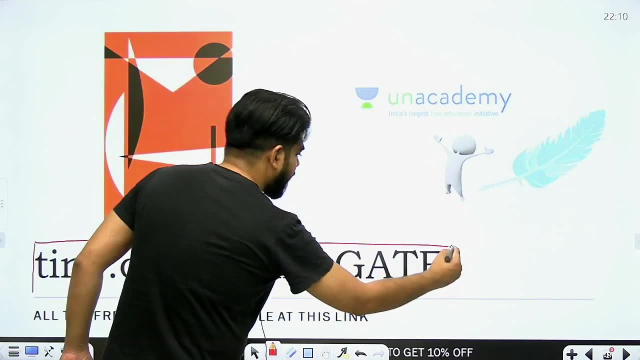 apart from that, this is my unacademy profile. on this unacademy profile, you should also follow me so that you can get the important updates of the unacademy also. right, and this is the notion page. You just have to type this tinycc slash vishal gate, so you will be redirected to a page. 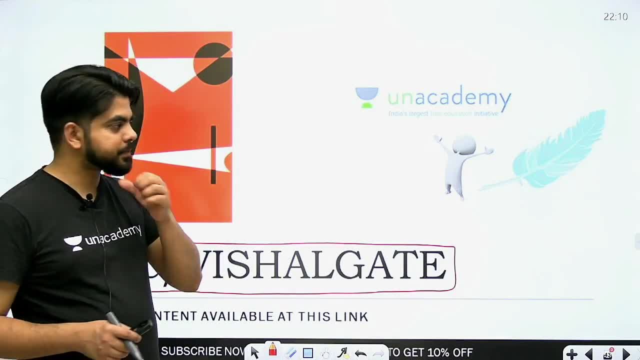 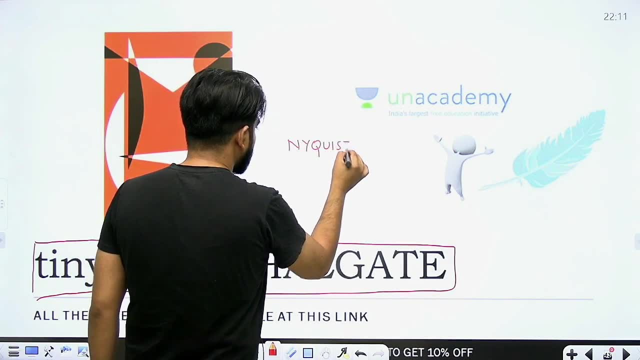 where all the special classes are arranged very systematically. so I have kept a lot of topics for special class, for example, Nyquist, Fourier series, latches and flip-flop double integrations. okay, lot of things, lot of things are there, so you will be getting all these. 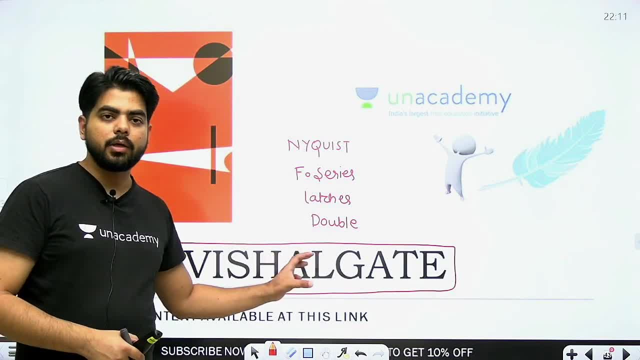 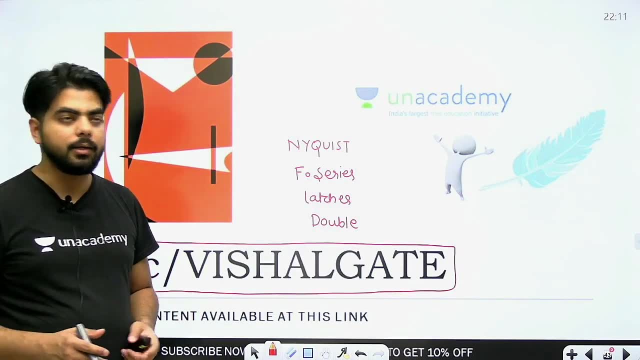 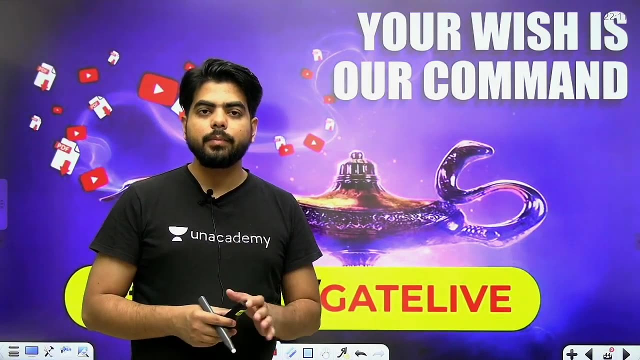 concepts, absolutely free of cost. You just have to type this in your URL. you will be redirected to that page and attend these lectures one by one. you will be getting a next-level confidence in these topics. that I can guarantee you. Now, this is the notion page of your YouTube, on which you will be getting the links of 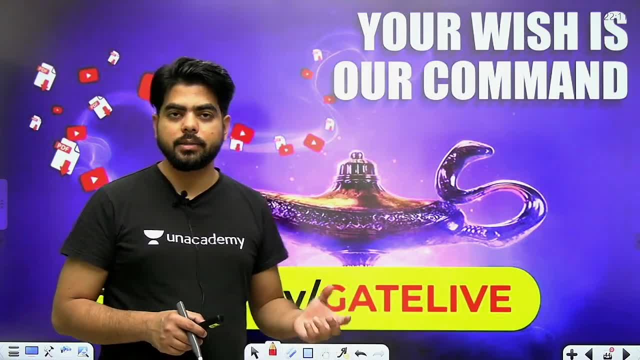 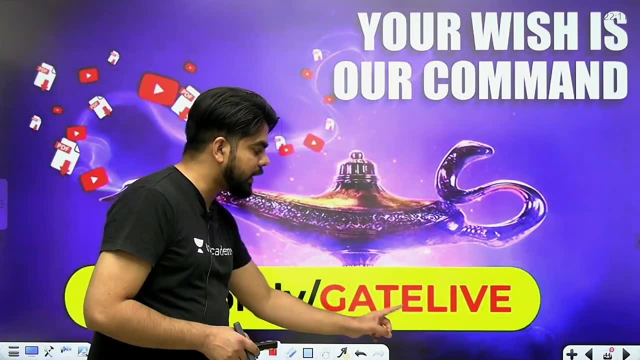 the YouTube. apart from that, you will be also getting the PDFs of that particular lecture, so this is very important for you, and just you have to type http dot double slash bit, dot li slash gate live, So gate live. You just have to type it in. 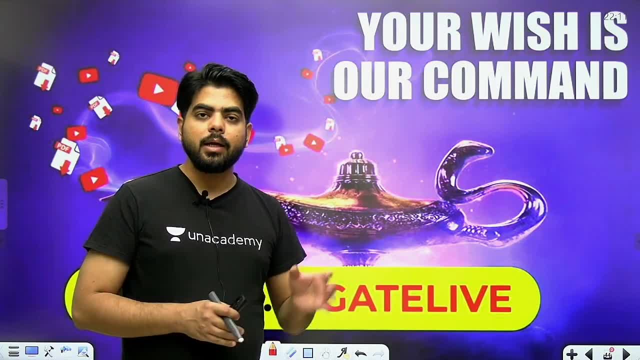 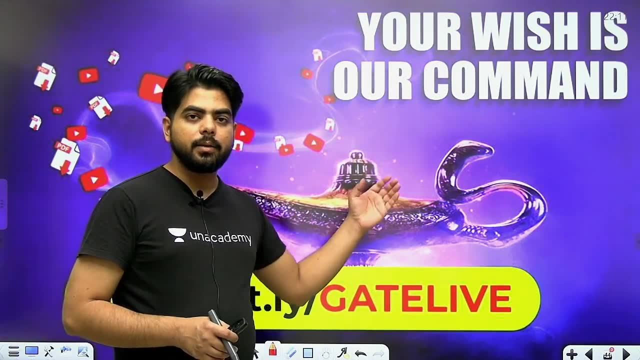 You just have to type in the capital so that you can access all the lectures. link and PDF are in systematically. So if you want to attend or you want to clear the examination with the free resource, then this is a channel for you. This is the best recorded videos which has been ever made. 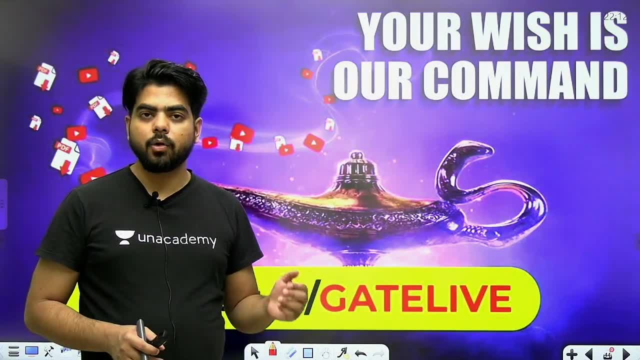 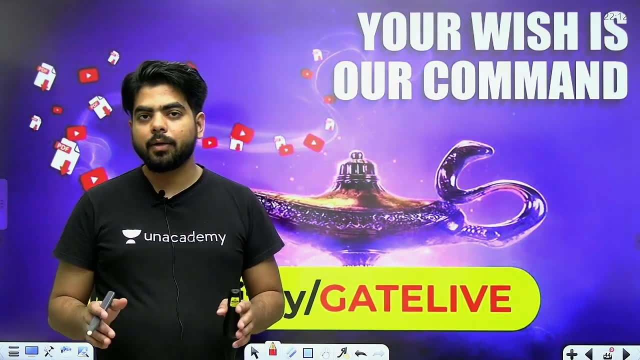 You just have to go to that lecture, Just click the link and download the PDF and start studying systematically. So we have also done this for you, so that any student, whether he is sitting any part of this country, should not face the difficulty in cracking the examination whether he can. 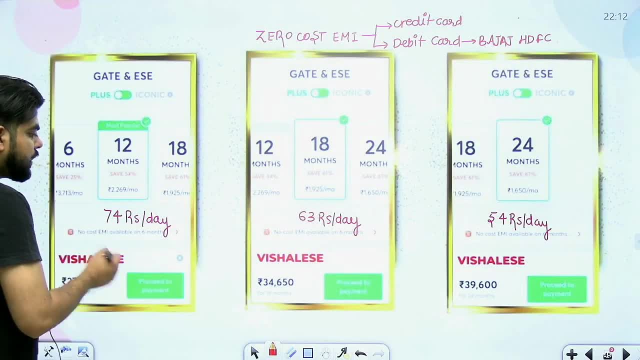 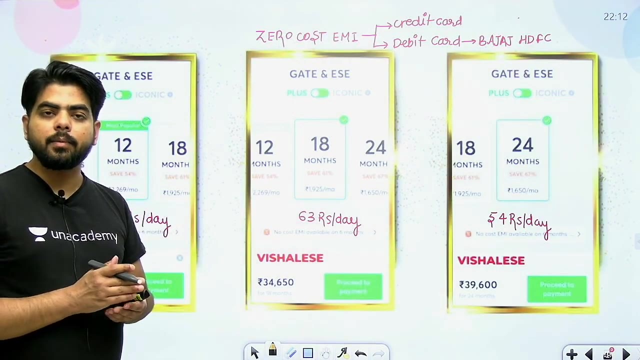 afford or he cannot. Now, if you can afford, then the subscription prices are not something which you cannot pay. it is very nominal amount which you can pay and you can just avoid all the distractions, all the time wastage which we will be doing in downloading those PDFs, arranging them, arranging 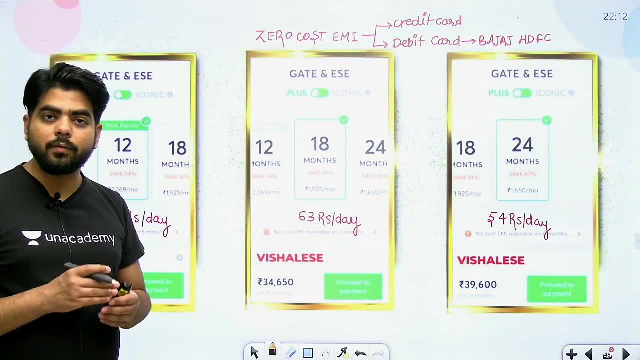 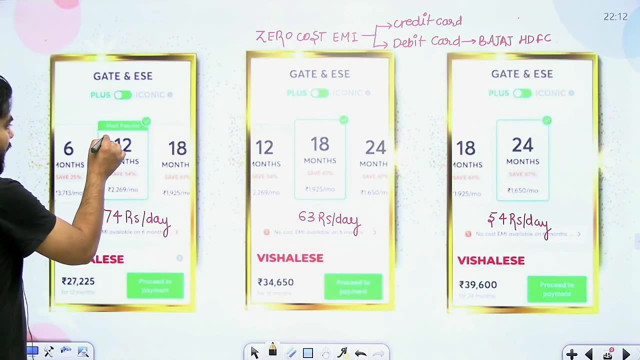 for the test series and a lot of other things that you have to arrange and doubt solving. so you have to arrange by yourself if you want to avoid all those distractions in a very, very nominal amount. so you can go for the an academy plus subscription for 12 months. subscription, You have to pay only 74 rupees per day. apart from that, for 18 months subscription, which is the best possible subscription, you have to pay 63 rupees per day. it is even lesser than the pizzas that you order on your home, so it is that much of amount that can shape. 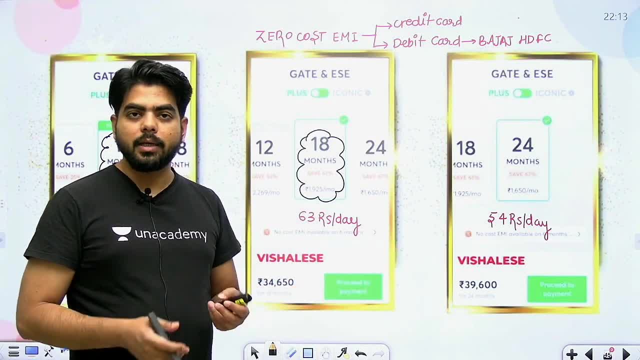 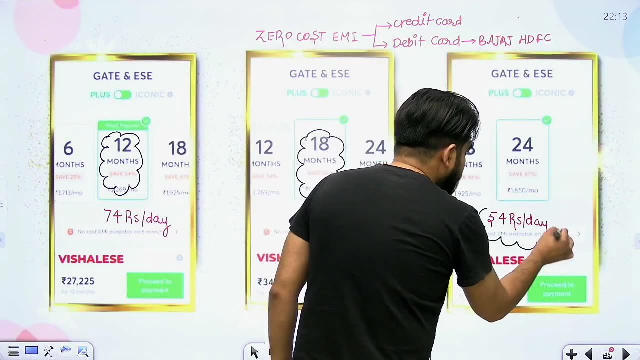 your career that can give you the best possible rank in the examinations under the guidance of the best teachers of the country, which has been right now placed on the an academy. Now, 24 months subscription will cost you 54 rupees per day. so these subscription amounts 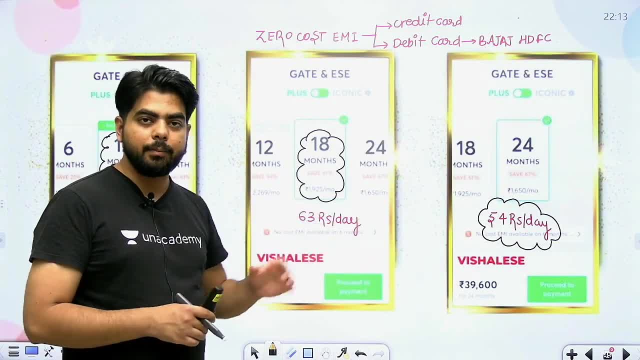 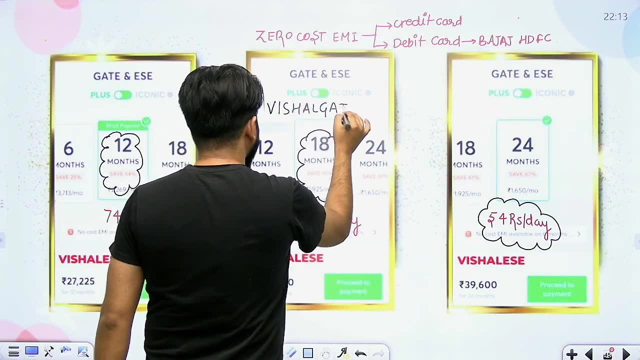 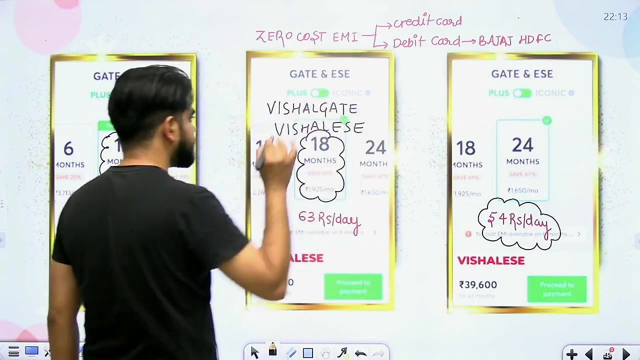 will give you the subscription for the desired period. apart from that, if you are using this code, you just have to remember this code. write my name, write gate after it. you can also write ESC after it. so you have to write my name and write ESC after it. so any one of these 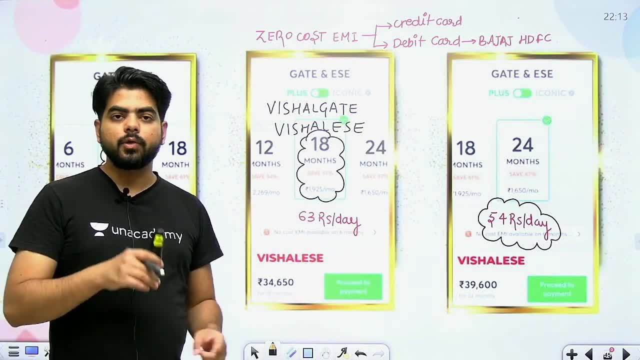 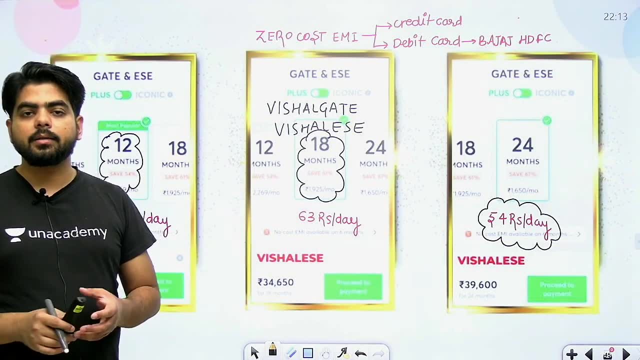 code. once you apply, you will be immediately getting the 10% discount. you will be getting all the features of the an academy. you will be getting the guidance of all the teachers present on an academy, and everything you will be getting. That is what you will be getting. 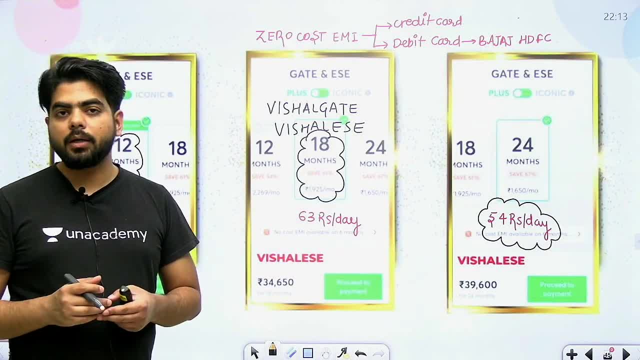 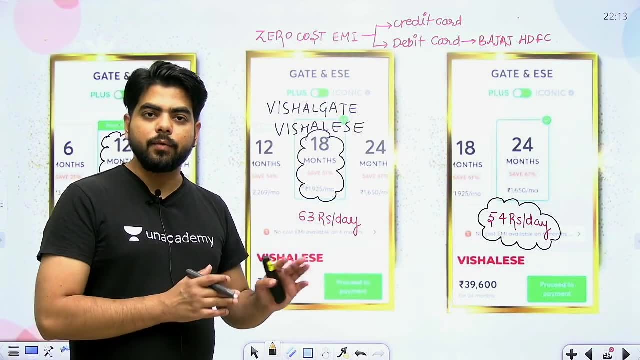 That is needed to crack the examination once you are using this code. so if you think we are working hard, we are giving our best content, we are giving the free content absolutely for you guys and everything that is needed for every student to crack the examination. so never forget to use this code whenever you are taking the subscription. so this code. is very important and you have to use every time you are taking the subscription. now those who are interested for the prices: total price amount. so let me tell you: total price is 27 to 25 for 12 months. For 24 months it is 39600. you can also pay this by using zero cost EMI. zero cost EMI can. 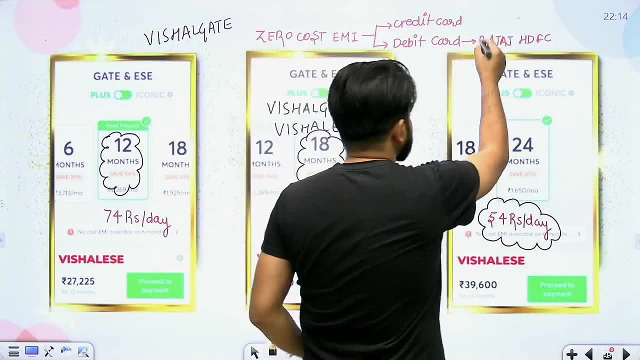 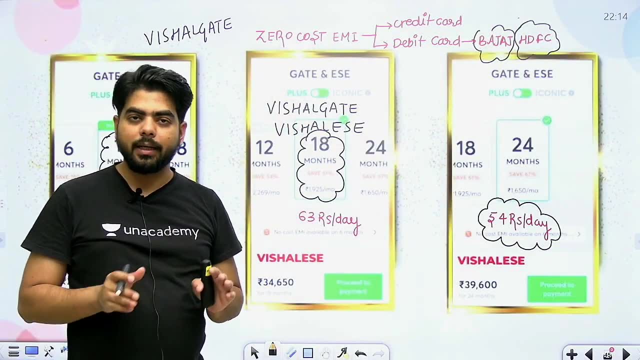 be paid by credit card and debit card. in debit cards, there are only Bajaj and HDFC as of now available. okay, so the zero cost EMI means you do not have to pay anything extra. any interest is not. you should not pay and you have to pay this much of amount on the daily. 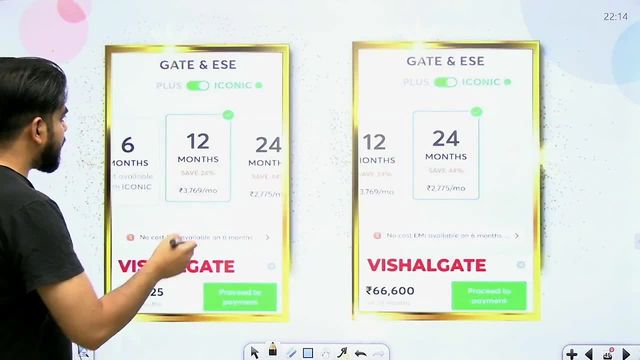 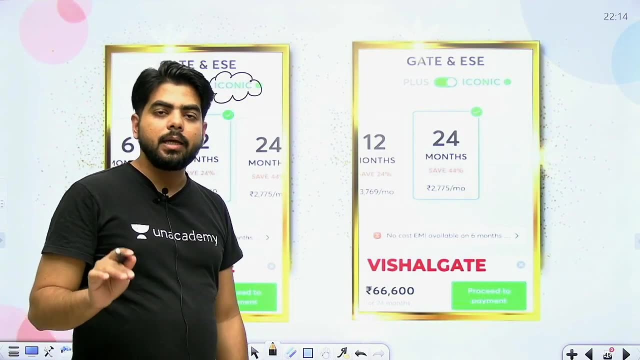 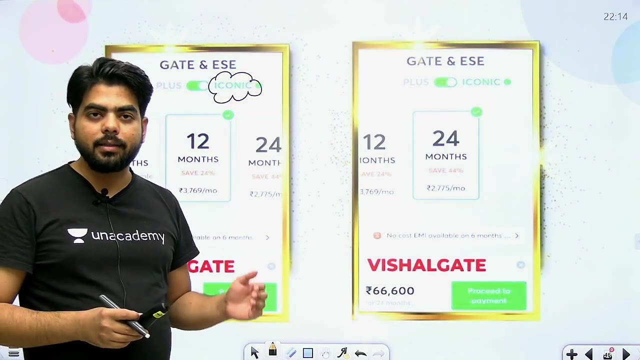 basis if you are looking for the zero cost EMI option. apart from that, if you are coming for iconic subscription. So in iconic I have already told you that your personal coach will be the game changer. he will be basically following you to give you the guidance so that you can get the success.